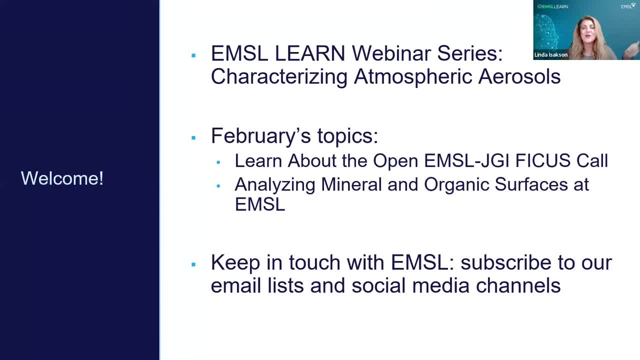 Wow, And Vancouver, Canada. So we are an international community. This is just amazing. Before we move on to the presenters today, I want to just briefly go over next month for EMSL Learn webinars. We have two in fact. One will be on February 9th and that one will provide information. 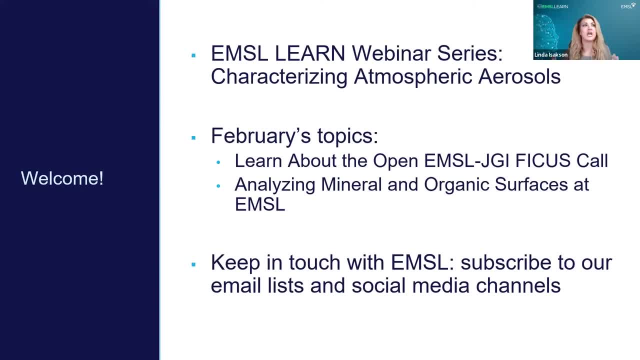 on the currently open EMSL Learn webinar. We have two webinars. One will be on February 9th and that one will provide information on the current EMSL JGI FICUS calls for proposal. If you are interested in submitting a FICUS call or a FICUS proposal this year, make sure that you attend. 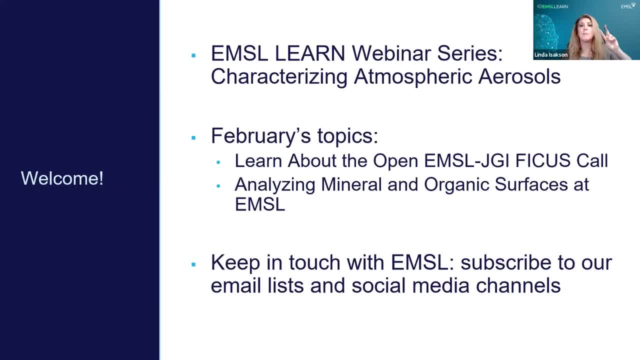 February 9th. The links for both of our open call for proposals are in the chat window at this moment, And our second EMSL Learn webinar is focused on analyzing mineral and organic surfaces at EMSL, And that one will be February 23rd And we hope to see you there too. Also, make sure to keep in. 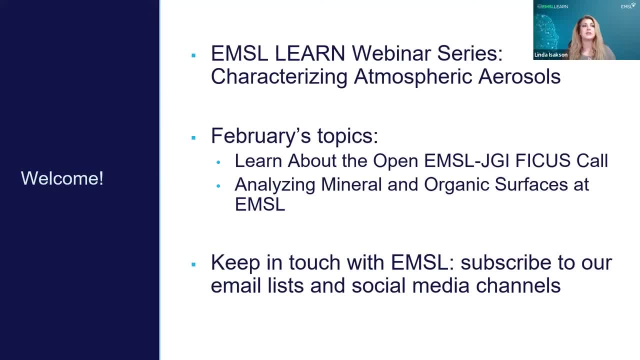 touch with EMSL by subscribing to our newsletter and our social media channels. if you haven't already, Again, links are in the chat for everyone. It's a really great way to keep in touch and keep up to date on our open call for proposals and other opportunities to work with EMSL, And so for. 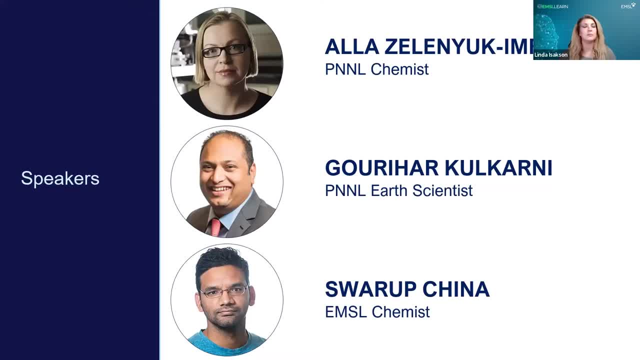 today we are going to be talking about the EMSL Learn webinar. And we're going to be talking about the EMSL Learn webinar And we're going to begin with PNNL chemist Alaa Zelenuk Imri. She is going. 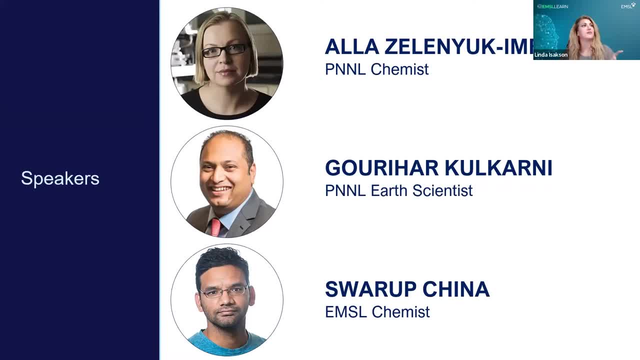 to be providing us with showcasing EMSL's unique single particle mass spectrometer for characterizing the physiochemical properties of individual particles. And then, after Alaa's presentation, Gorhar Kulkarni, a PNNL Earth scientist. he's going to be talking about the 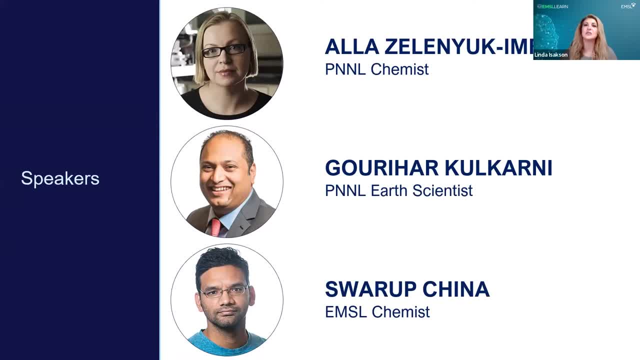 EMSL Learn webinar, And we're going to be discussing our custom-built ice nucleation chamber for in-situ studies on the ice nucleating properties of atmospheric particles or aerosols. And then, lastly, we have Chaurub China, who is EMSL's chemist, And he will be presenting on how EMSL's 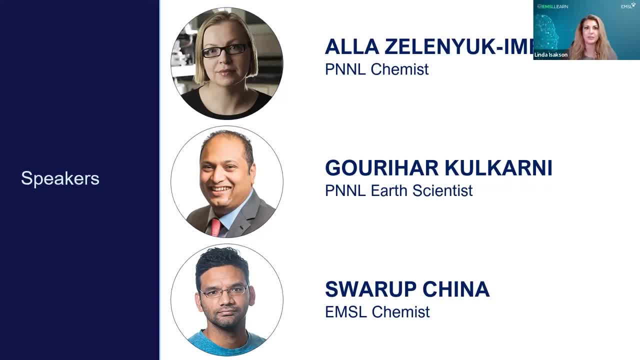 microspectroscopy and mass spectrometry capabilities were used on collaborative projects And he's going to be talking about the EMSL Learn webinar And we're going to be considering ab우, one of the responsibilities that were funded through the eMSL, and arm the. 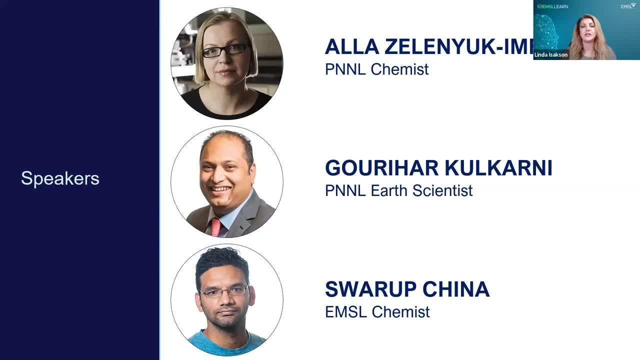 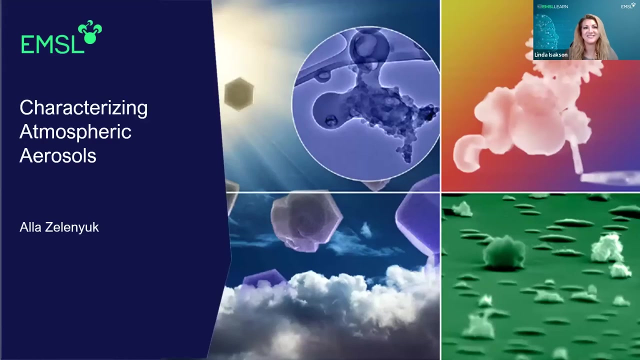 Atmosphere Radiation Measurement user facility through that user facility proposals, and so after the presentations we will have a quick q&a. So if you have questions, make sure to drop them in the chat And we will discuss your questions afterwards. And with that I turn it to Alaa. 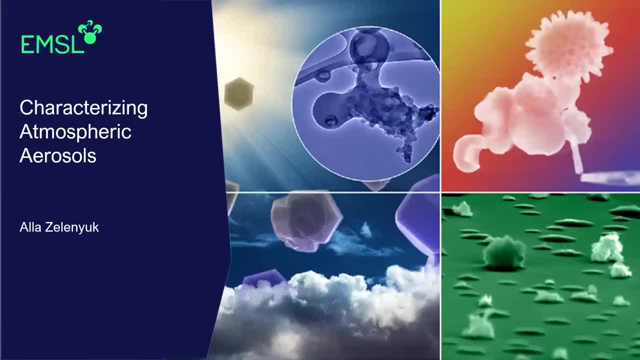 Thank you, Linda. Hi, I'm Aliza Linuk and today in this webinar, we will discuss a variety of different instruments and tools which we have here at EMSL and which are available for all EMSL users to characterize atmospheric aerosols. 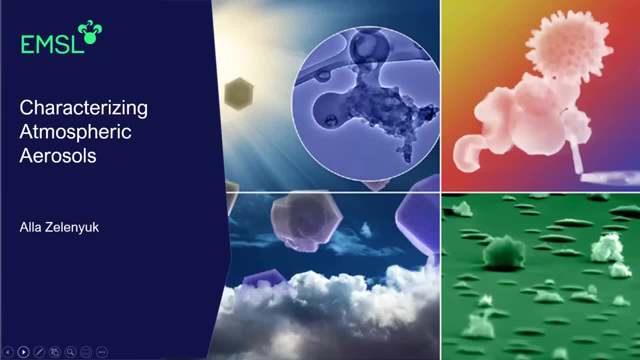 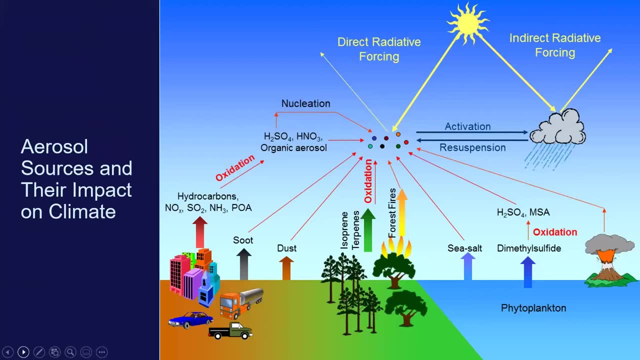 And I will start with a very brief introduction of why are we interested in properties of atmospheric aerosol particles? And the answer is very simple: In the air which we breathe in. they impact our health, visibility. they impact climate, both directly, by absorbing and scattering solar radiation, and indirectly, by activating as cloud droplets and ice crystals. 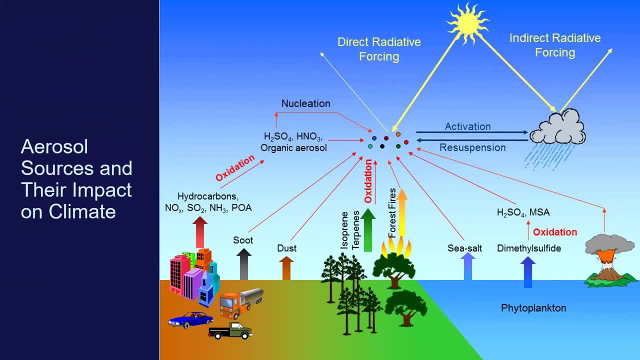 Particles come from many different sources. Some of them are natural, Like sea salt, volcano eruption dust particles, while others are related to anthropogenic activities. They're coming from emissions from combustion, cars and biomass burning. They're coming from industry. 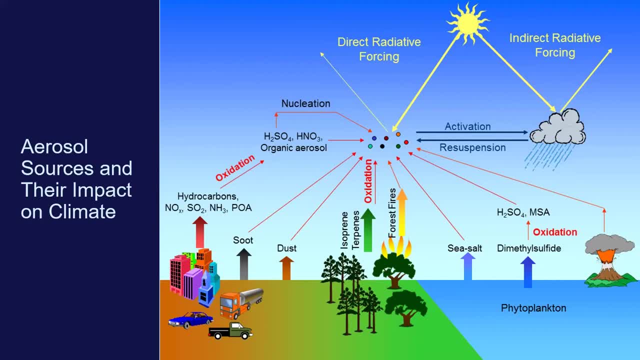 And some particles, like sea salt or dust, are directly emitted- We call them primary aerosols- while others are formed in atmosphere by oxidation of gas-based species emitted by trees and by industry. We identify aerosols as both subject and Present thinks of them as such, as a. 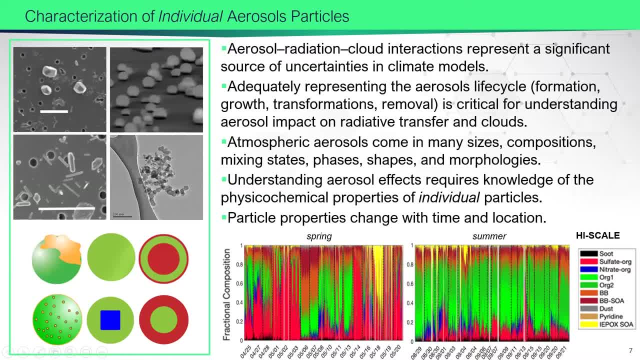 Aerosol radiation, climate and the problemsЧ At present are also still with variations- of how ourusu Those types of particles and in order to understand how they impact, mostly how they and climate, climate And at present Ra And at present Ra. 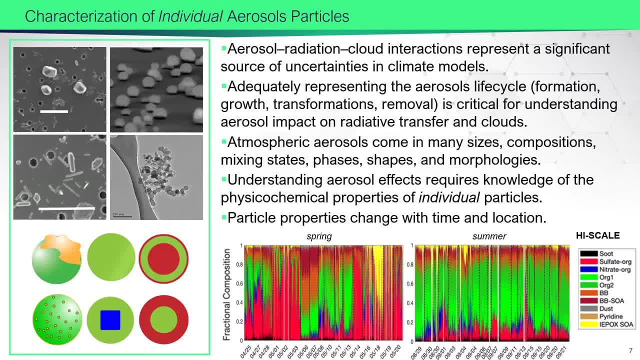 in climate model And to understand impact of aerosols on both radiative transfer and clouds. it is critical to properly represent aerosol life cycle, understand how particles form, how they grow to climatically relevant sizes, how they transform during aging and transport. 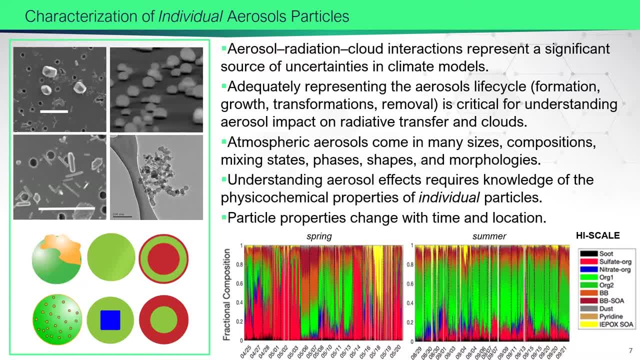 and how they eventually removed, by wet or dry deposition and or by photolysis. And what makes this task is very challenging is that the fact that atmospheric aerosols come in many different sizes: composition, mixing state: what comes with what on different particles? 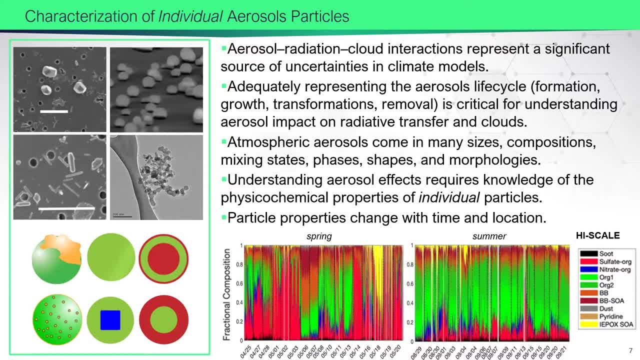 phases, shapes and morphologies. Here you could see just a few examples of particles which were collected on micrographs or cartoons of particles containing secondary organic aerosols, shown here at the bottom, And particle properties also change with time and location. Here at the bottom. 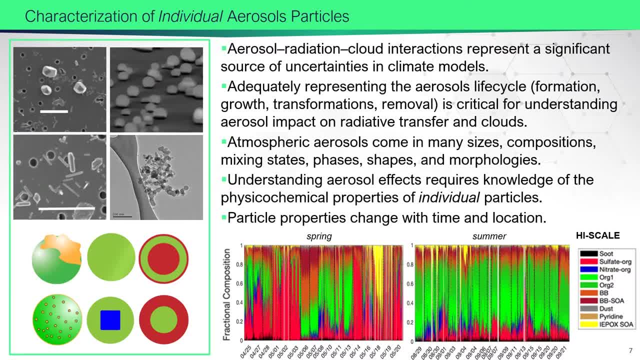 example from high-scale field campaign which took place close to our SGP site, which shows that, depending on season, depending on different days where we fly, on time of the day, altitude, types of particles are changing and the impact on climate also will be very different. And 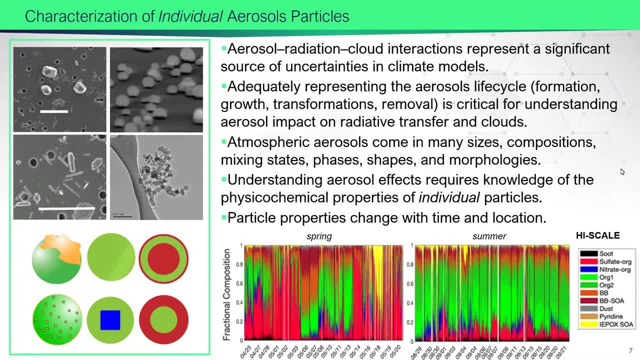 what we found in this study is that all types, nearly all types of particles which we characterize, contain different amount of secondary organic aerosol. So ideally, what we want to do is to look at one particle at the time and to tell you how big it is, what it's made of, what its 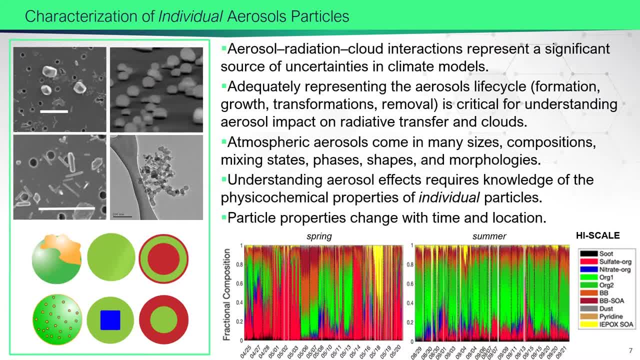 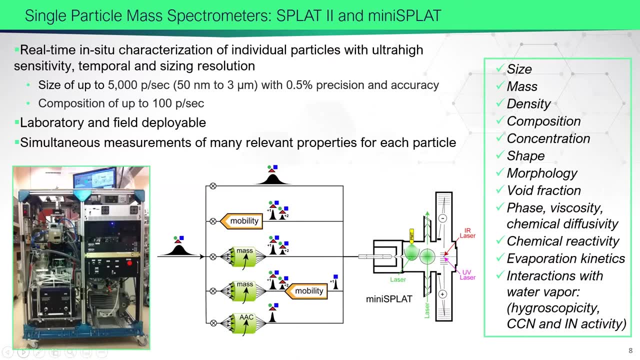 cloud activating activity is what optical properties are, And to do it we develop our single particle mass spectrometer. We call it a single particle mass spectrometer, We call it araploid. I'm having trouble clicking it. This is my radioprocessor, a splat tool, and it's miniaturized version, mini splat. 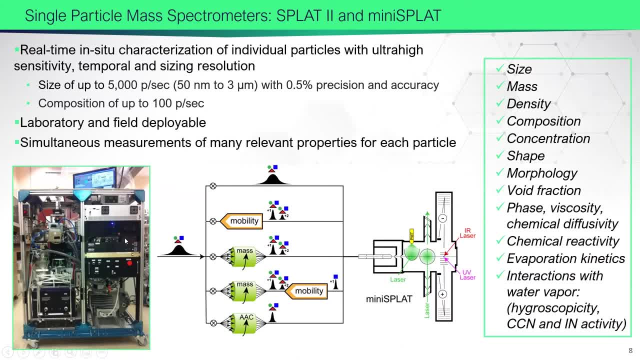 shown here on this photograph. These instruments are available for deployment both in the laboratory and in the field, including on board of aircraft, And they make it possible to look at one particle at the time, in situ and in real time, and to tell you, even if the paper is really small and that the data that 계post was coming from recent photographs. But understanding this data we speak of very quickly, but, for example, any vendor, for example, would need a flash as possible, a very useful device In my case, I don't need to remember. And then we found some aspects that here in the 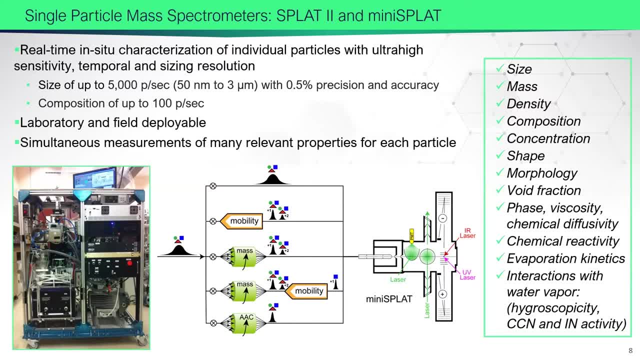 details list, and they don't have to change it. And so, of course, you have to provide a very typical how big it is and what it's made of, and we can do it with very high sensitivity, very high temporal and very high size and resolution, and this very high sensitivity also makes it possible to look 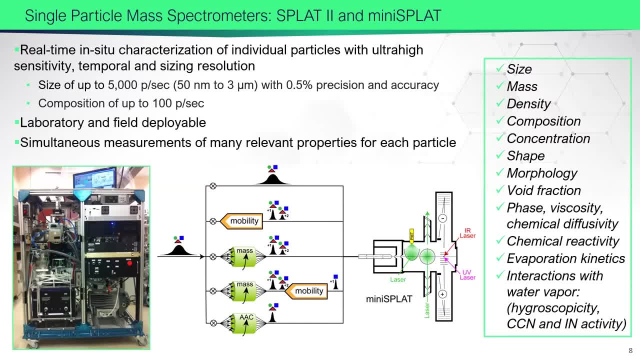 not only at all particles but also at size and mass selected particles and determine many other particle properties listed here on the right, and I will illustrate many of these measurements in my talk, and I would like to point out that many of these measurements are done as part of EMSL user. 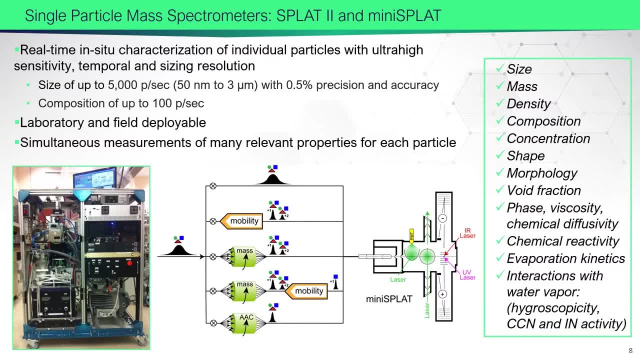 proposals and in this approach, which we often term multi-dimensional, single particle characterization, not only we could learn a lot about individual particles properties, but also about relationship between different particle properties, including RSL, size dependent composition, CCN activity, OIN activity and reactivity. 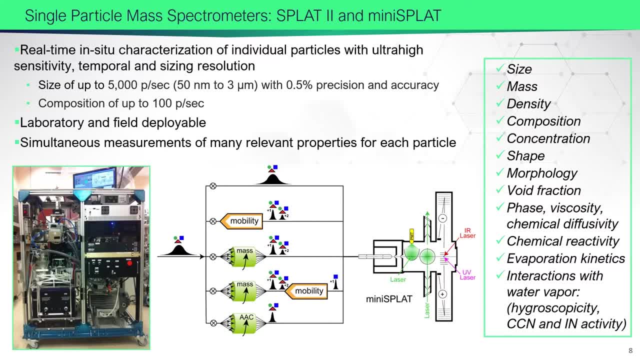 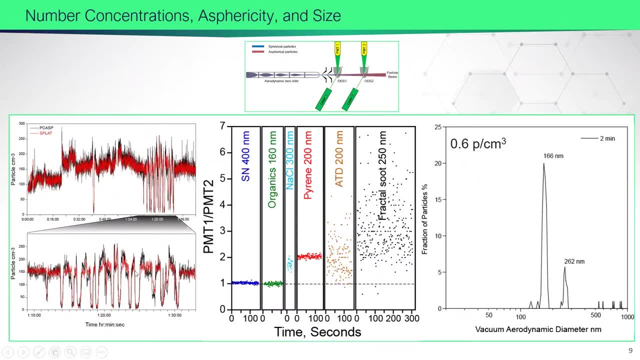 So let's start with first example where we measure using our single particle to measure particle number concentration. with one second resolution you could see here we'll fly in and outside the cloud and measuring particle number concentration, particle sphericity, which depends on particle composition and shape. it's very important also to quantify measurements by single particle mass spectrometer. 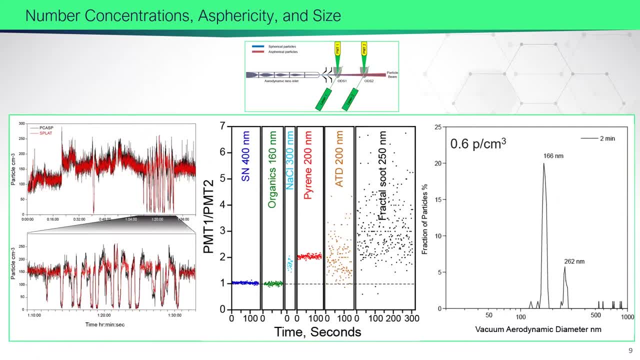 and account for composition and shape dependence. And then transmission efficiency and particle measurements of particle size, distribution here number concentration by less than one particle per CC and we detected it in two minutes and it's very important for some studies, like for example for ice nucleation, for understanding particle ice. 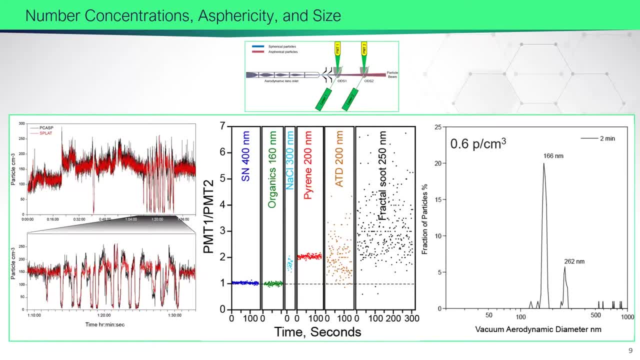 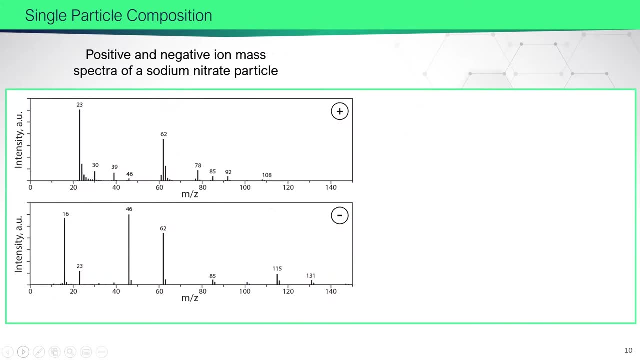 nucleation activity where concentration of this very special particles which activate as ice nuclear is extremely low. When we look at properties of size, selected particle as particles goes goes on, sorry. we determine particle mass spectra. we looked at positive and negative mass spectra and quantify composition both of 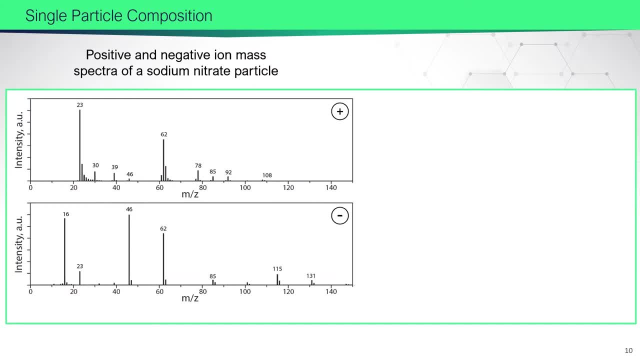 volatile and non-volatile in each fraction of each particles. And we do this measurements in the lab. we could find, tailor our ionization approaches and characterize in the composition of entire particles, as shown here. we could drill inside and look what is on the surface of the particles, what is inside, or we could look or only at volatile fraction of particles. 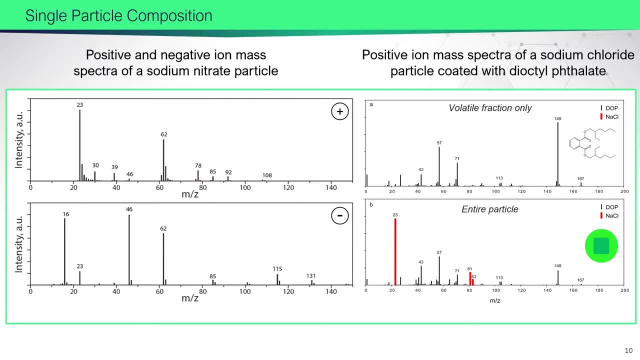 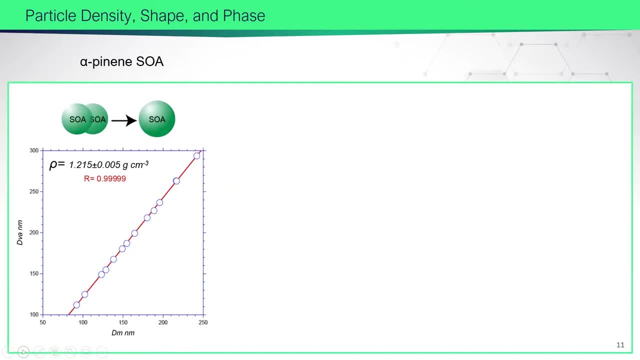 So different ways to quantify particle composition. when we looked at size selected particles, we could measure the additional properties like particle density, very important when we tried to convert size distribution into mass loadings or calculate yields of formation for species like alpha-pinene, SOA or any other types of particles. 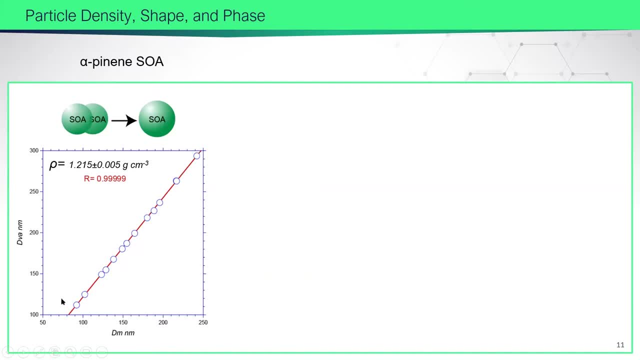 Here you could see high-resolution measurements of density for alpha-pinene SOA particles. We find these particles as spherical and measure their density with very high precision and accuracy. We also show how condensation of SOA on the surface of cubic sodium chloride particles. 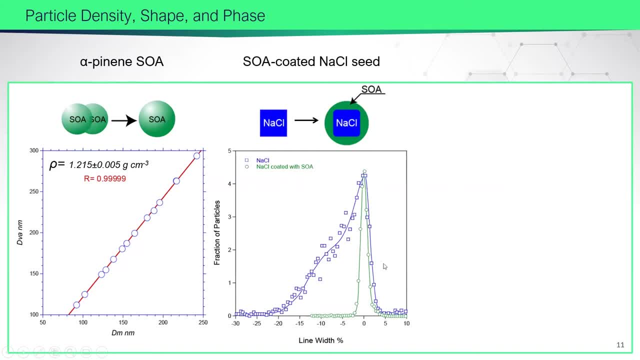 convert these particles into spherical And we could determine it by looking at the shape of this line width. And for highly spherical particles like soot, we measure their fractal dimension, measure their mass in fractional femtograms, could determine the size of this primary agglomerate which 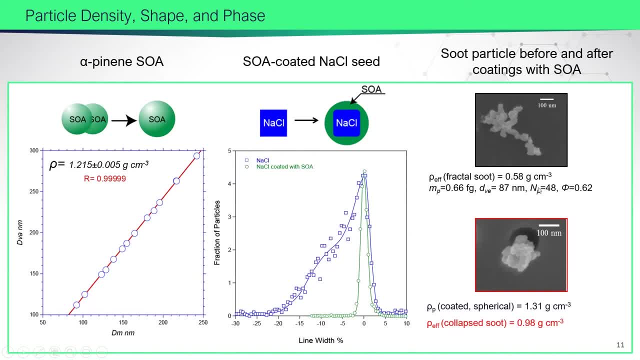 makes this fractal structures: number of these agglomerates per aggregate of different size or mass, void fraction, And then we could monitor changes in shape of these particles as we deposit different coatings, in this case SOA. We see these particles becoming spherical. 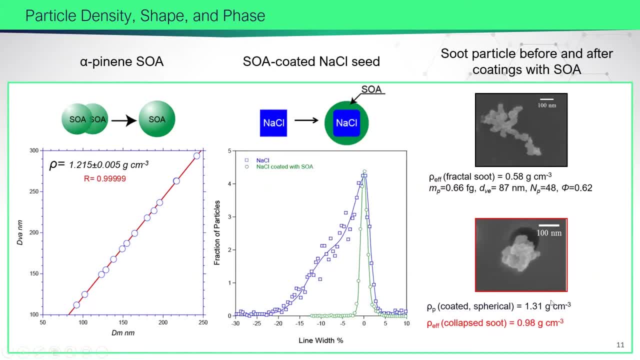 Their density is changing And after removal of these coatings we find that soot collapses and has very different affected density, void fraction And, as GK will show in his presentation, their isonucleotide properties are changing and their optical properties are also changing. 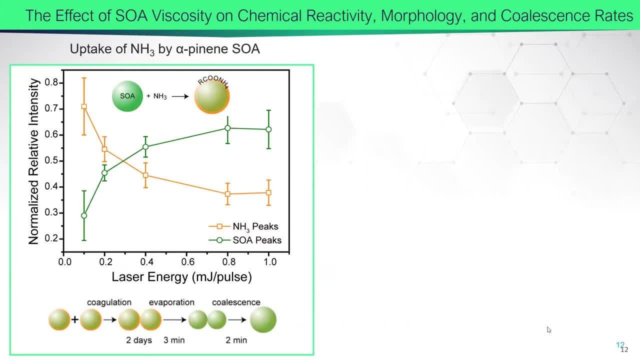 Particle viscosity and other properties which we are measuring is another very important properties which affect aerosol chemical reactivity, morphology and coalescence rates. In this study we characterize uptake of ammonia by alpha-pinene SOA particles And what we show is that this exposure results. 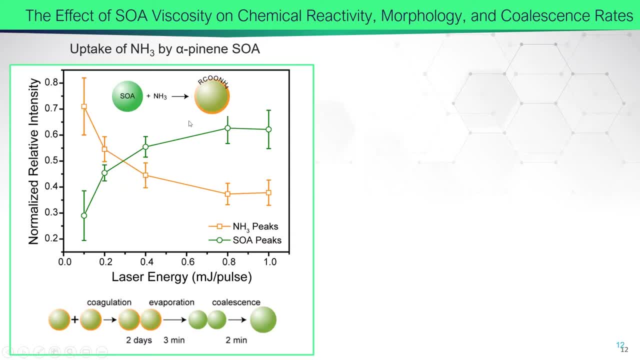 in formation of very thin- 4 nanometer thin layer on the surface of SOA particles And this very thin layer completely shuts down, causing a very fast ammonia uptake. And when two of these particles coagulate, they do not coalesce and remain as spherical. 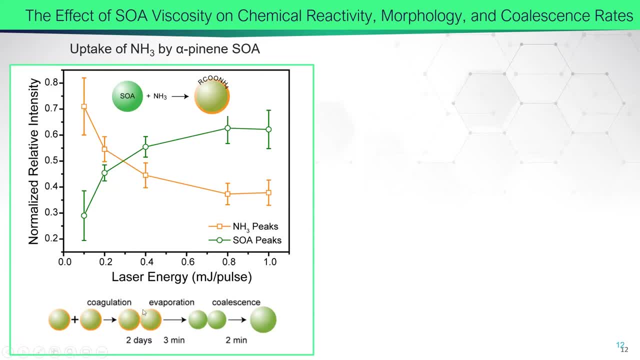 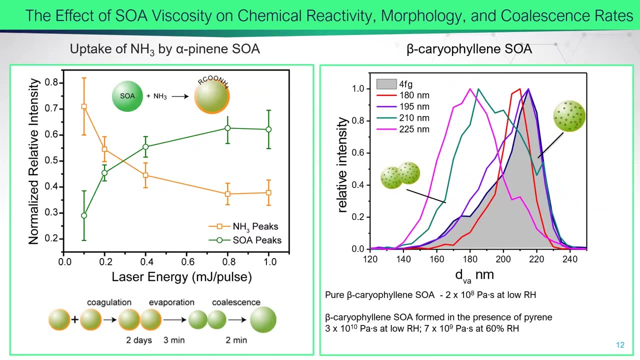 kind of doublet particles for over two days, But when the semi-volatile layer evaporates, this particle coalesce on the time scales of two minutes, which allows us to calculate viscosity of these particles and follow their faster transformation. Another system which often exhibits this: 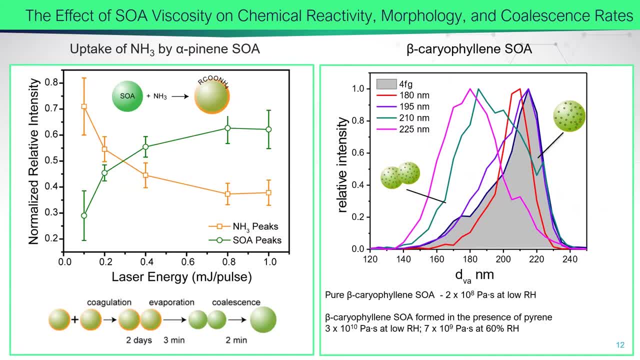 coagulated but not coalesced particles are other types of SOA. They are more viscous, like beta-chlorophyllene SOA. In this case, particles with the same mass could be spherical or could be just spherical doublets. 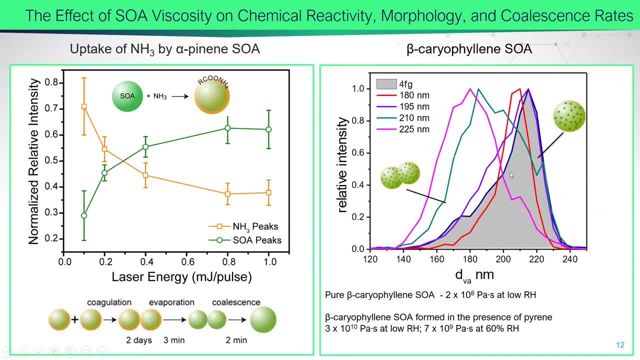 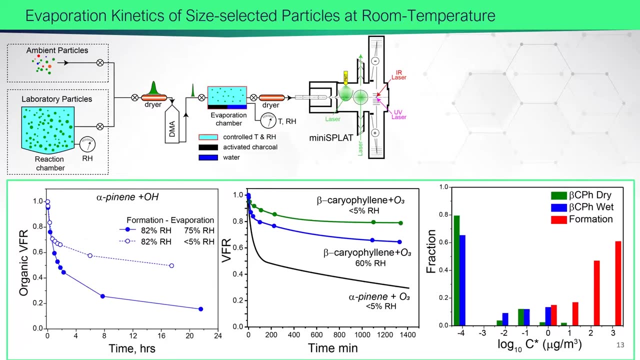 So with our approaches we could separate these two different types of particles And just watch how, when these spherical particles coalesce at different relative humidity and measure their viscosity as function of relative humidity. It is also important to understand volatility of atmospheric particles, to see how much they will shrink. 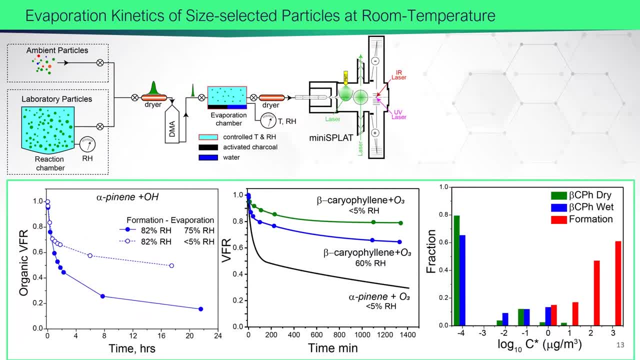 how long they will survive when they're transported far away from the sources. And we do it by this approach, which we developed in my lab, to measure evaporation kinetics of site-selected particles at room temperature, which allows us to avoid thermal decomposition, which 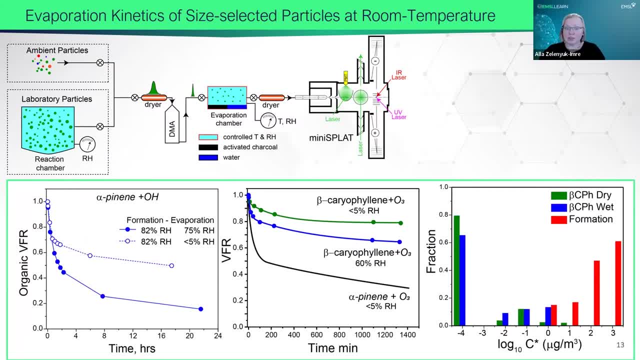 is a problem in some of the experimental approaches. So in this approach we're looking at volatility at both low and elevated relative humidity, which allows us again to separate these issues of particle volatility and viscosity And, for example, for beta-chlorophyllene. 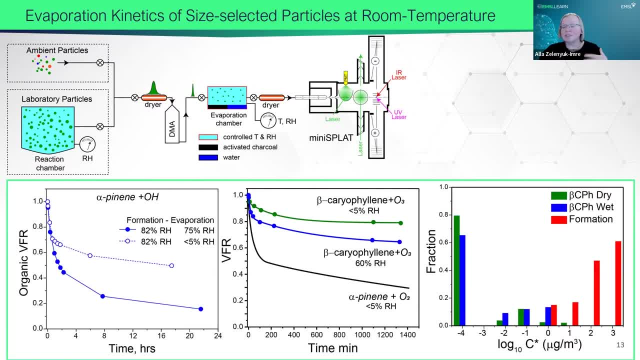 we find that not only are these particles more viscous, they also have significantly lower volatility compared to alpha-pinene And from these measurements we could extract volatility basis set. It could be incorporated into model. It shows that incorporated into model results in significantly better agreement. 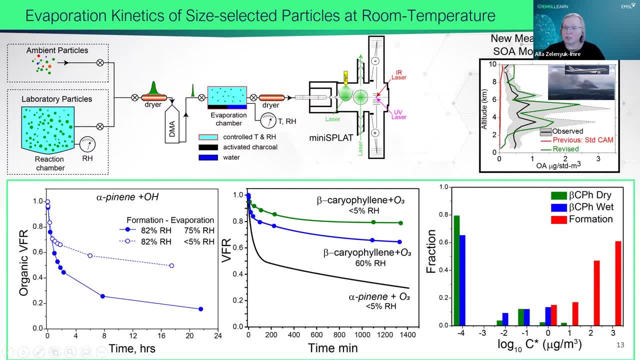 between measurements and model compared to previous climate model prediction. And I also would like to point out that we do these measurements both on laboratory particles and on ambient aerosol, either by deploying instruments in the field or pulling particles through the inlet through emerald roof. 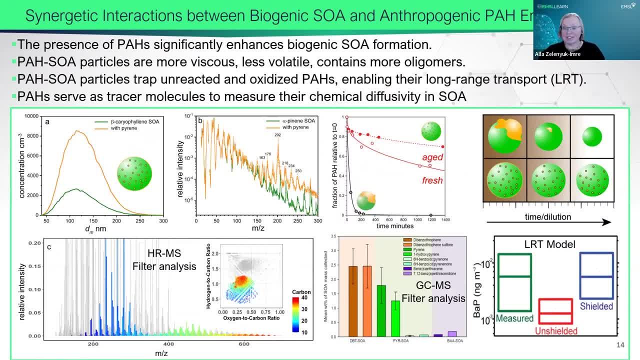 Just another example of actually several user projects, both from MTU, PNNL and Oregon State University, which focus on synergetic interactions between biogenic secondary organic aerosols and anthropogenic emissions like toxic polyaromatic hydrocarbons. 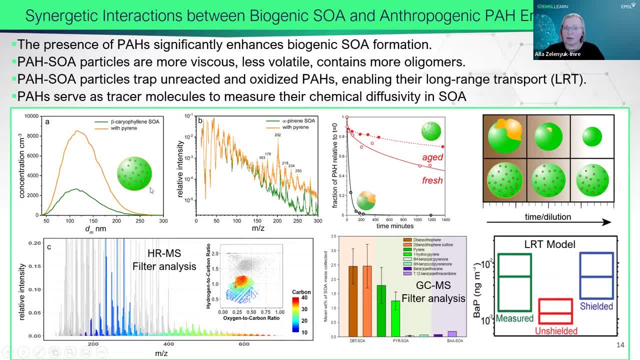 These measurements were done both in real time at AMSOIL. We look at enhancement in formation due to presence of these pHs, their composition, higher fraction of ligamers. We could follow diffusion of these polyaromatic molecules within particles and measure chemical diffusivity. 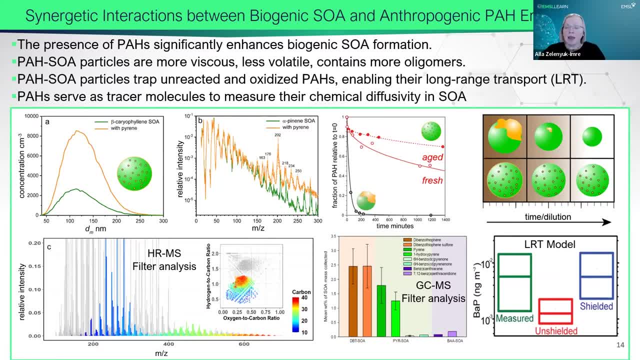 another measurement of particle viscosity And we also collect these particles on substrate for offline analysis. This was done in MTU, high resolution composition analysis and GC-MS in Oregon State, And also these findings about trapping and shielding of these toxic molecules was incorporated. 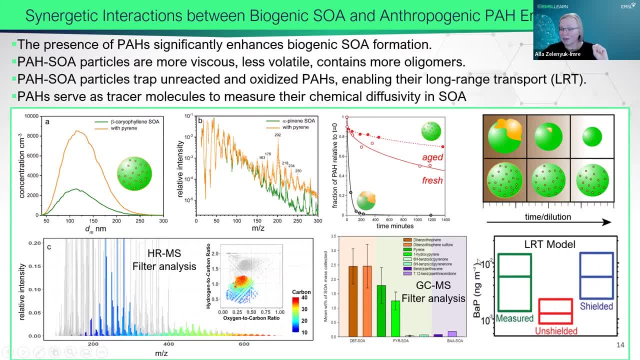 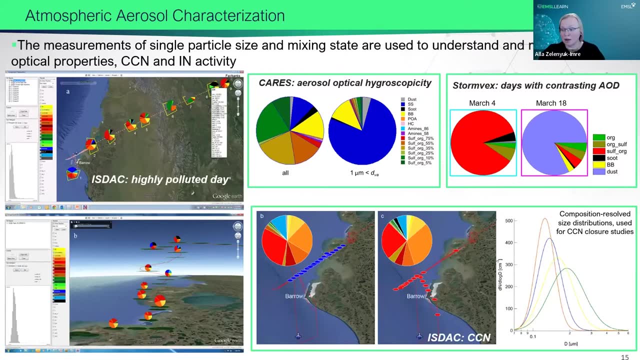 in their long-range transport model. And again we obtained significantly better agreement with measurement compared to previous approaches. And finally, just a few examples of field measurements. Here we are using our single particle measurements of particle size and mixing state to understand. 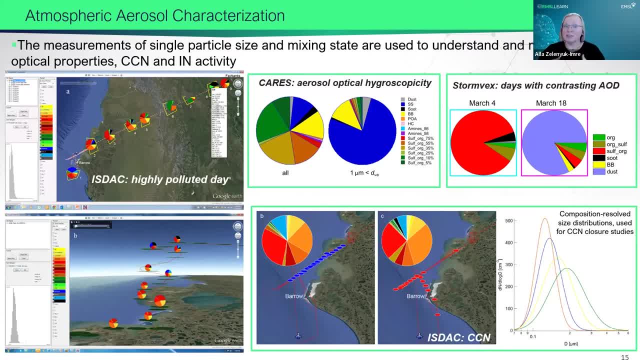 and in many cases to model aerosol optical properties, CCN and IN activity. For example, in Storm Peak Lab we explained days with very high aerosol optical deaths by long-range transport of dust from Asia to Colorado In California. we show that very small fraction. 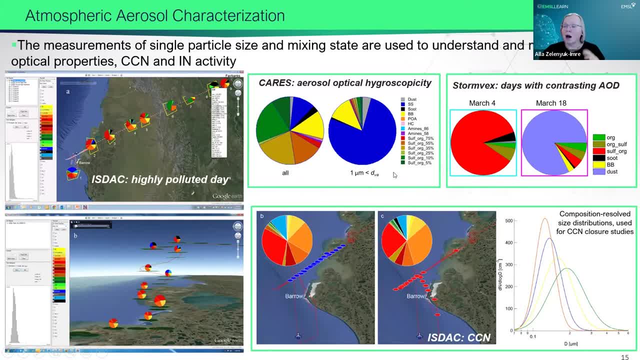 of sea salt, which are super micron, are responsible for 80% of light scattering signal versus all. absorption signal is explained by OK As much smaller particles. we could follow particle composition along airplane track and look at changes in particle composition size distribution. 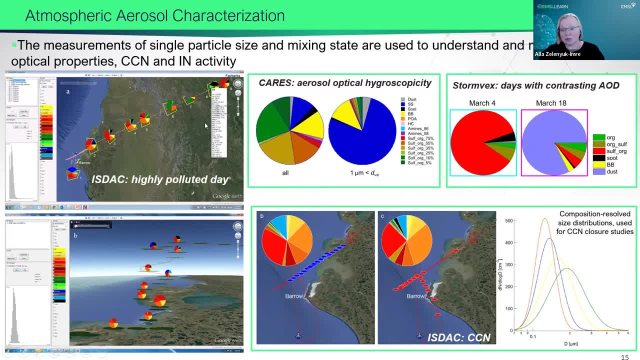 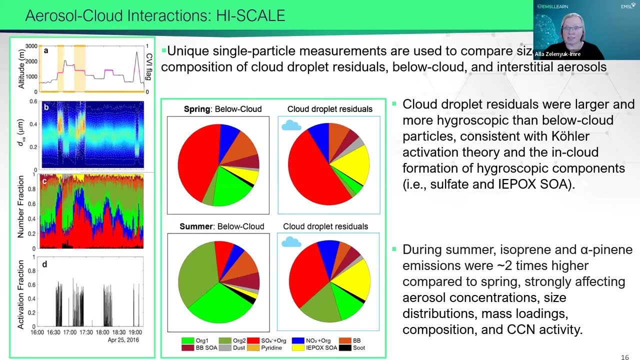 and all other observables which are measured on airplane plane and also look and model CCN properties of aerosol by using their composition, result, size, distribution and conduct CCN closure. Here just another example of CCN measurements from high scale, where we find that cloud droplet. 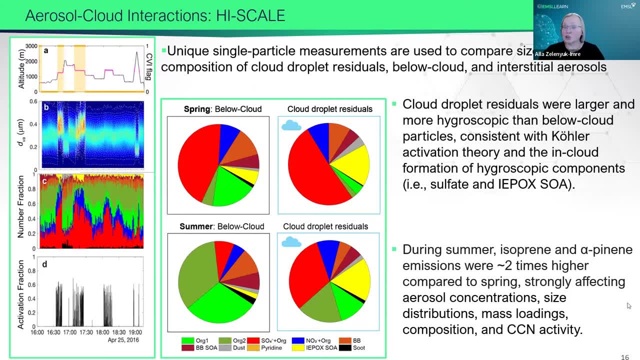 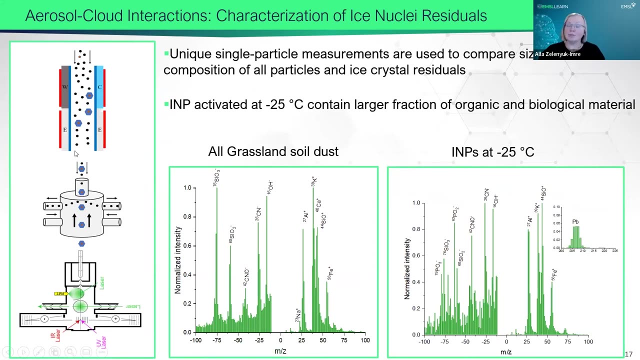 residuals are larger and contain much more hygroscopic material like sulfate nitrate and epox-SOA, consistent with color activation theory and in cloud formation of this species. And finally, my last examples compares properties of soil dust particles which enter AMSOIL: custom ice. 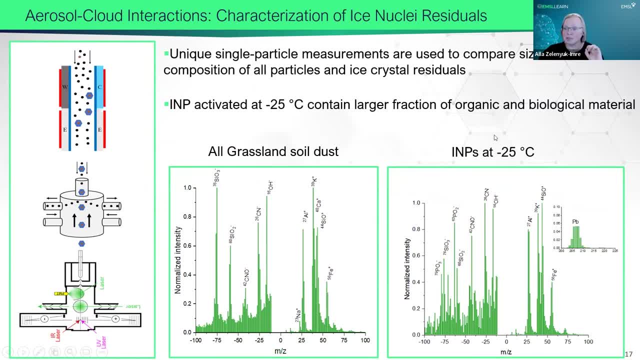 nucleation chamber And those very, very special ones which activated at warm temperature, at minus 25 degrees. What we find? that ice nucleating particles contain significantly higher fraction of organic and biological material compared to all grass, soil, dust which enters this ice nucleation. 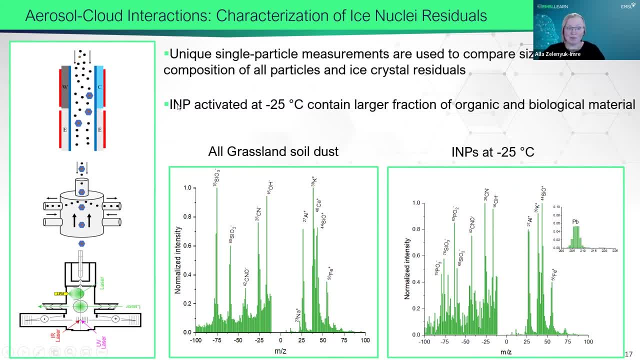 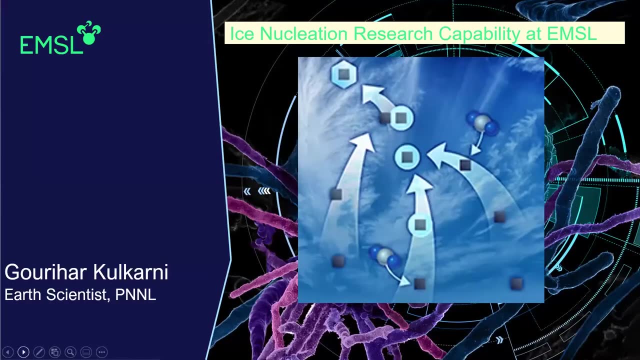 chamber, And with this I will pass it to GK, which will describe measurements by this custom ice nucleation chamber in much more details. Thank you, Har crush, Thanks, Hравla. So I'm going to discuss the ice nucleation research capability. 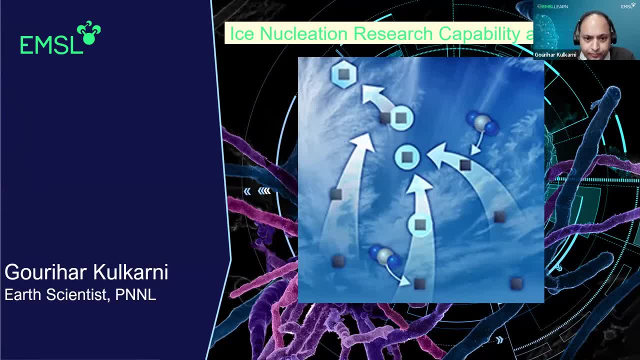 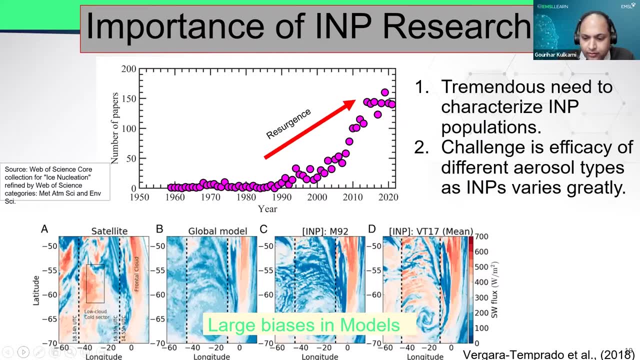 available for the users at AMSOIL. Before Let's see forward. So before let me quickly highlight the importance of today's, the importance of today's research And finally, let me emphasize just one particular fact. It's just one of the ophiocyanin radios Foods that VeganDrop, KingできNonore and Can 나. 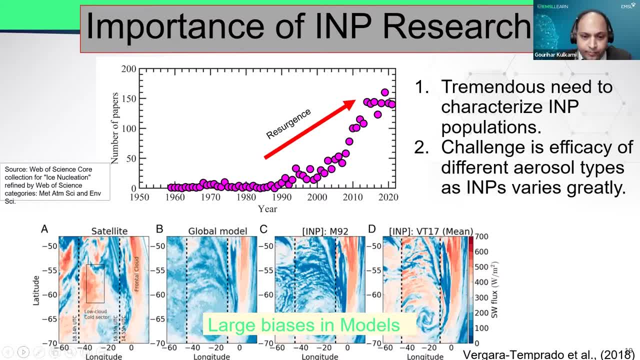 of INP research. Here I'm showing an example where the number of papers published in the under ice nucleation category and you can see that from last 10 plus years there's a tremendous growth in the number of papers published, showing that the you know efforts going on in this area. 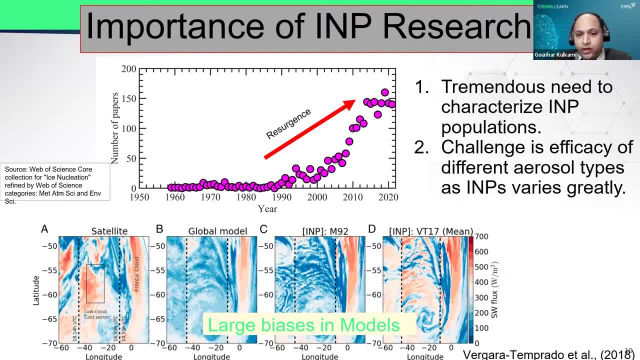 and the reason for that is a twofold. One is the just that we don't have enough measurements, especially there is a need to characterize the ambient INP population, and second one is that we haven't really understood the why certain aerosol types are more efficient compared to others, For 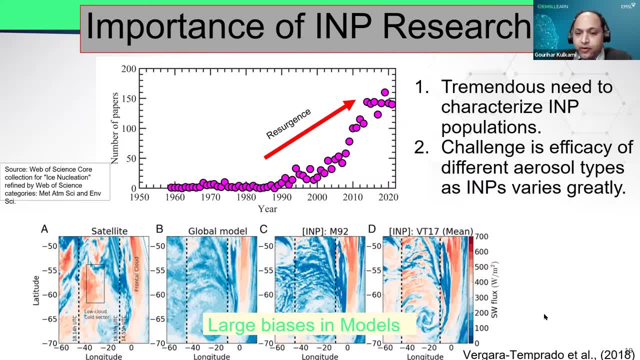 example, the efficiency of the dust particles are better than the soot particles, and we haven't really understood that part, and so this poor understanding has reflected into the poor representation in a model, And you can see at the bottom here a comparison between the observations and the modeling. 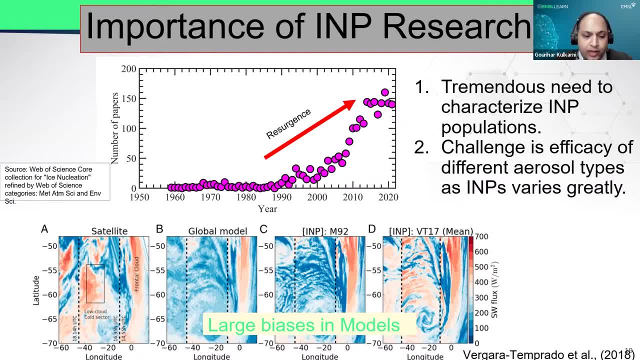 results. The panel A shows the satellite observations of the flux from the ice containing clouds, versus the panels B, C, D shows the the model results, and you can see that they are different. So how you can improve this further, I'm not able to. 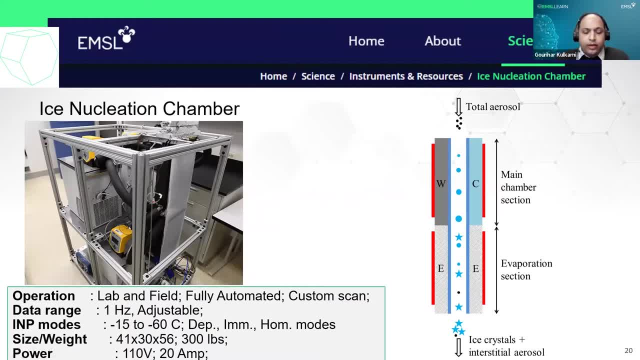 There you go, So the EMSL. we have this ice nucleation chamber Shown here on the left. It has an aerosol inlet at the top, and so the a cross sectional view of the chamber is shown on the right. So the aerosols enter at the top of the chamber as they enter the chamber in the first part. 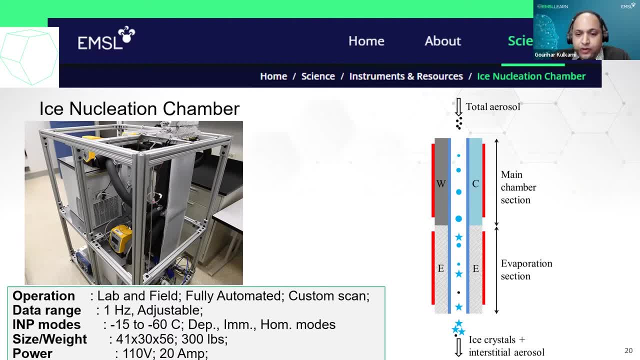 of the chamber. they are activated into droplet, So we call them a supercooled droplet because the temperatures are below zero degrees C. And then those droplets are activated into droplets, So we call them a supercooled droplet because the temperatures are below zero degrees C. 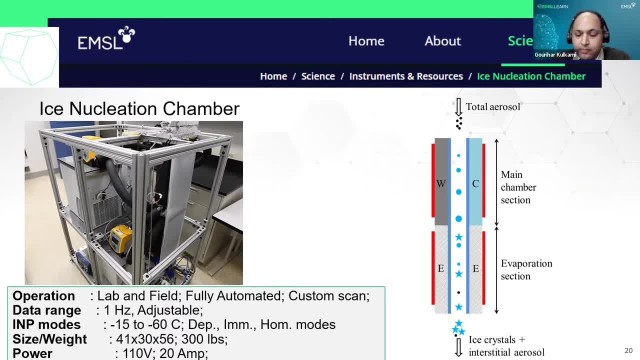 And then those droplets are activated into droplets, So we call them a supercooled droplet because the temperatures are below zero degrees C And they are exposed to different temperature conditions like minus 20, minus 30 degrees C in the evaporative section, and that's where the droplet freezes and the droplet which did 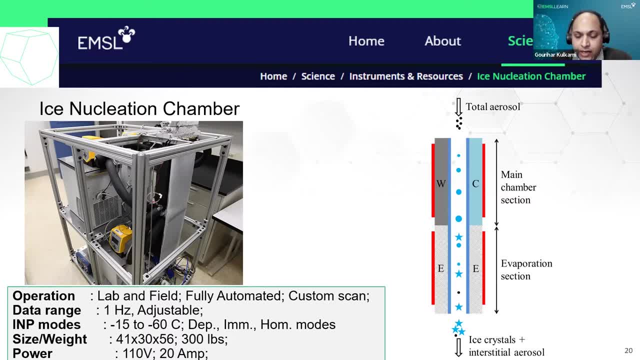 not freeze, basically evaporate or shrink. So at the end of the chamber you have an OPC instrument which basically counts the number of ice crystals, And so, using this information, you can calculate the frozen fraction or the onsets. the table here on the left. 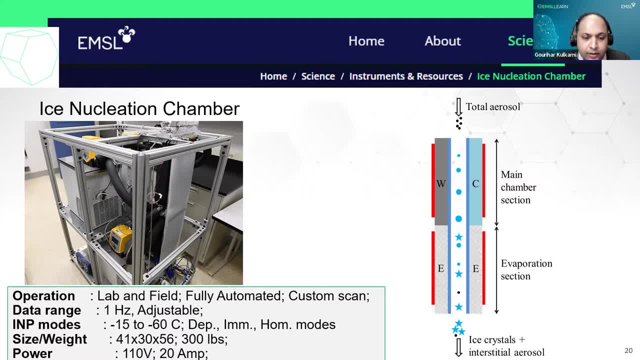 Here's the ice. here shows the specifications. Chamber can be deployed in the lab as well in the field. It's a fully automated. The data frequency is one hertz or you can adjust that as well as the. you can go the deposition or immersion or homogeneous freezing modes in the. 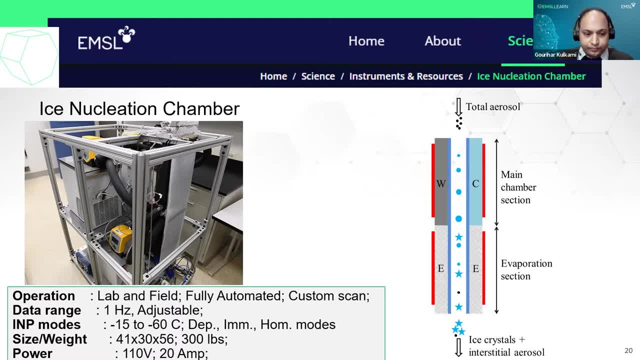 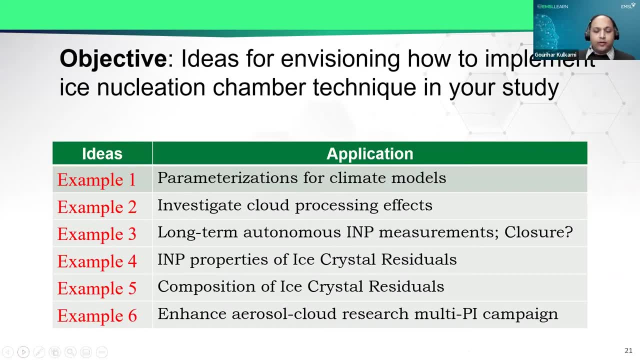 chamber which are highly relevant in the atmosphere. So here are some ideas regarding the application of the chamber. Starting with, you can run the chamber to develop the parametrization for a cloud model and all the way till you can separate the ice crystal residues and look into the composition and the morphology. 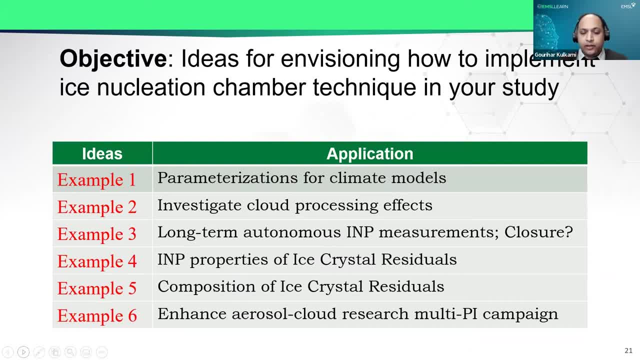 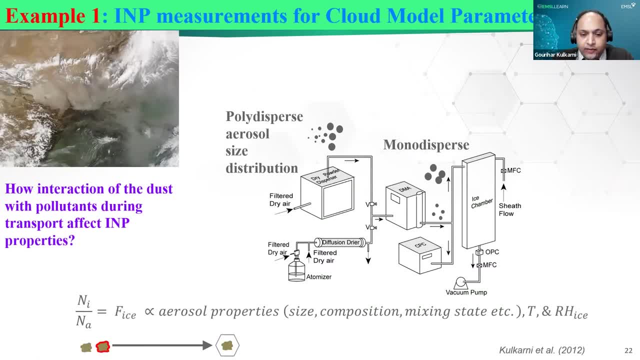 of them And let me go through each example at a very high level. So in this example you can generate the different type of aerosols and investigate their INP efficiency. So you can generate the polydispersed size distributions, or they could be mono-dispersed. You can dry disperse or you can wet atomize and what you 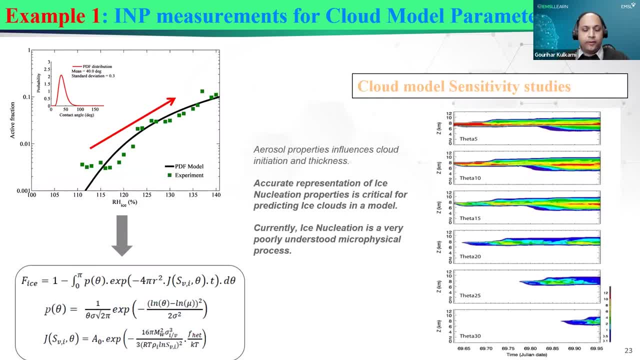 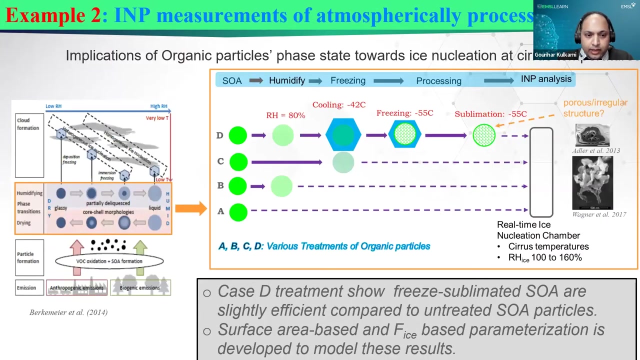 can do, then, is you can use this data to either develop the new parametrizations or constrain the existing parametrizations, and then you can feed those parametrizations into a model to understand the the sensitivity of different experimental parameters on a cloud field. In second example, here you can modify the inlet of the chamber to investigate the effect of 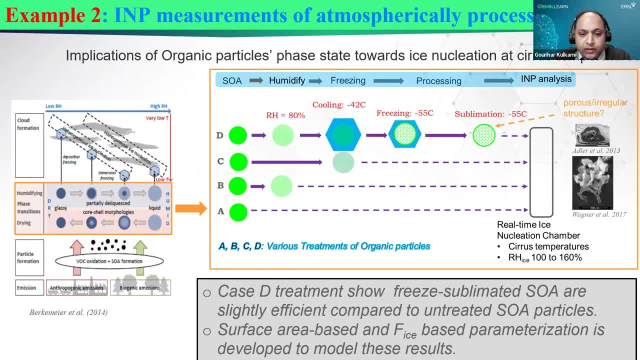 if you treat the particles versus the, if you untreat the particles and you can compare. So here you can see the example of organic particles which are humidified, then free, sublimated, and you look at the INP efficiency of those treated particles and compare against the unrated. 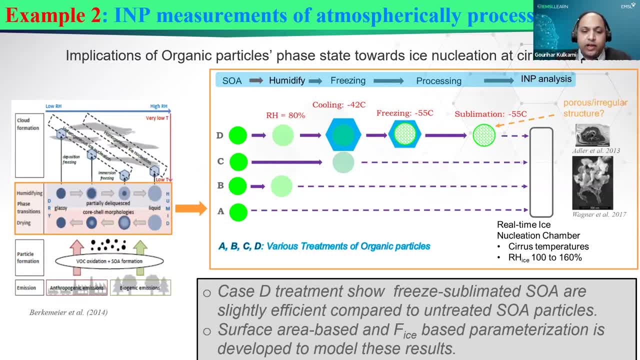 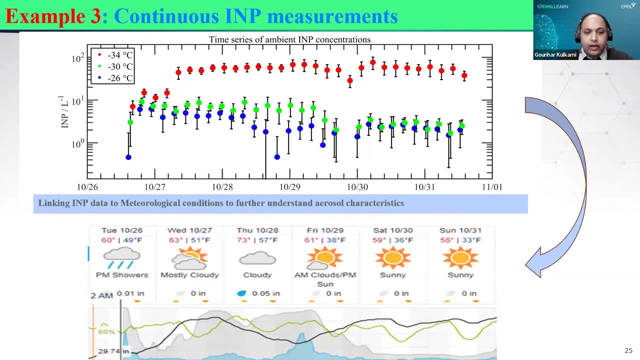 particles. just then you'll understand more about what aerosol properties actually affect the INP efficiency. And basically the idea here is, in simplified way, is to you are simulating a individual aerosol particle trajectory of that in the atmosphere Before the chamber can be run autonomously. and here I'm showing you the the time series of 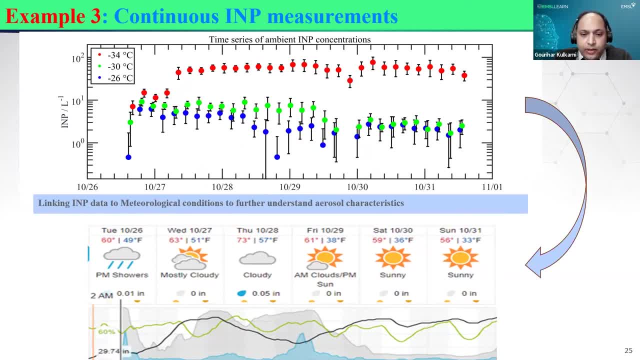 ambient and peak concentrations at three different temperatures, and what you can do with this information is you can connect this information or link this information to the meteorological conditions, like a wind, clouds, the temperature, humidity and also, if you have any co-located site distribution or the composition or the morphological information. what you can do is you: 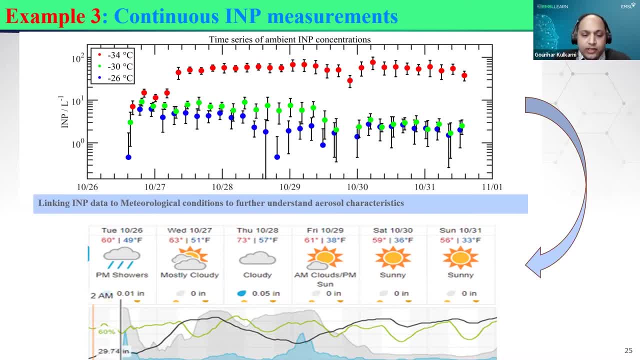 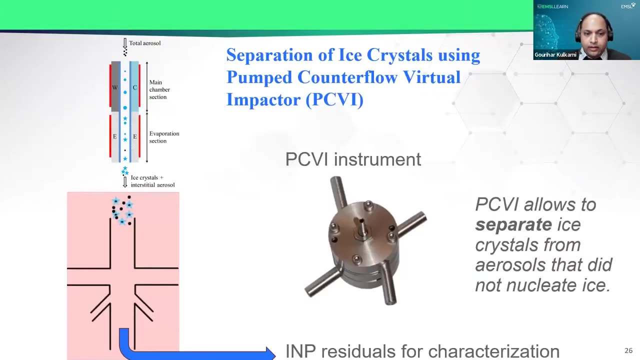 can do what you call the INP closure. So such studies are very important to develop the parameterization for a model to represent the ice containing particles in the cloud model or climate model. So another instrument that you can connect to the at the bottom of the chamber is the 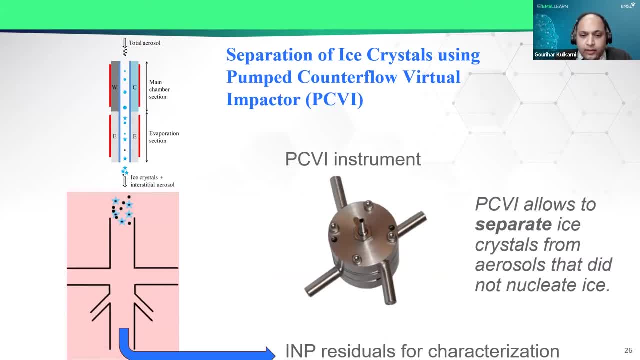 IRP. It's a very tiny instrument but very powerful. that what it does is. it allows you to separate the large ice crystals from the interstitial particles, the particles which did not declare ice. So I'm going to show in a small movie here. so what you have is at the end of the 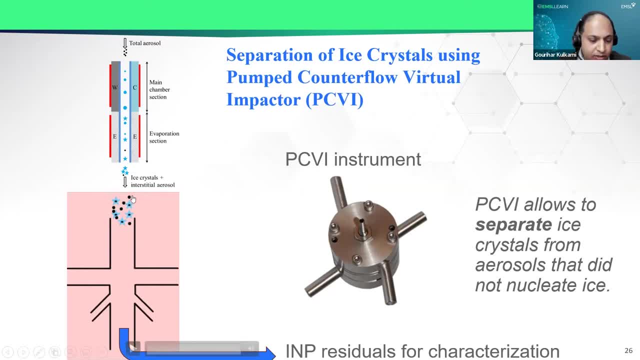 chamber is the mixture of ice crystals and interstitial particles and in this movie you will see the in a simplified a working principle of it is and what is the doing is basically you can separate the ice crystals from the interstitial particles and these ice crystal you can. then you can crack open these ice crystals and you have the residues and 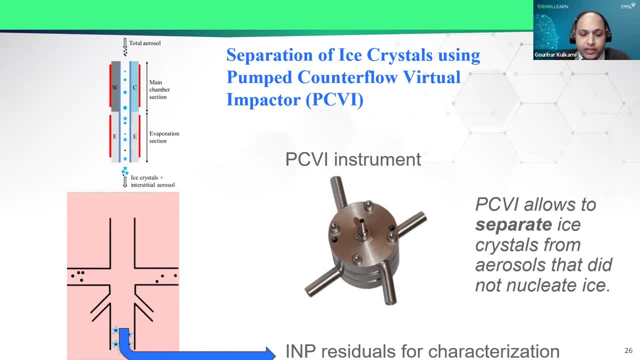 they're going to send those residues to mass spectrometers or in a single particle composition analysis instruments to look into what is so specific or what is so special about those individual particles that nucleated ice compared to the particles that did not the ice. So you can do a lot of things once you have a PCVI hooked up to the chamber. 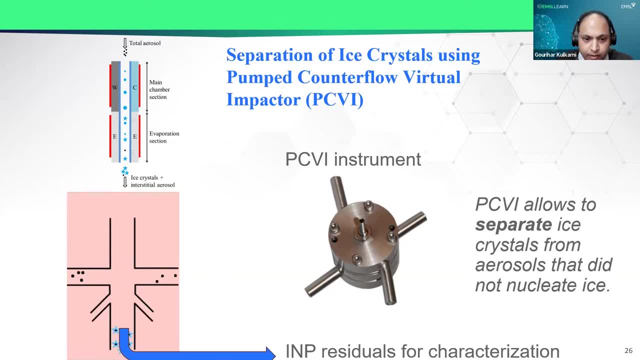 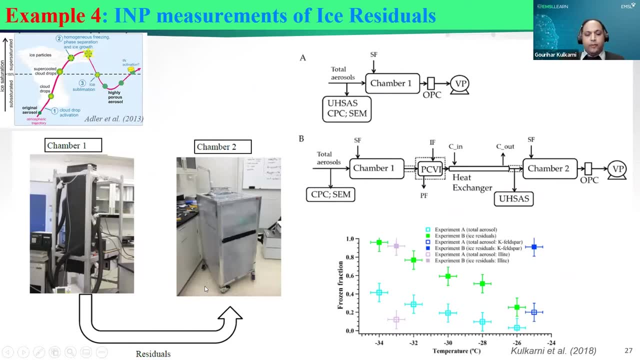 Here's an example. Let's see. Okay, so here's an example again about the PCVI application showing you you can connect the two ice chambers in series. So idea is that you have residuals coming from chamber one and you transfer it to the chamber two. 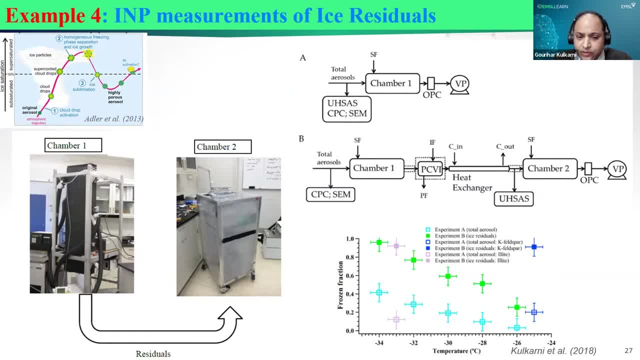 and look at the ion efficiency. It's a very powerful tool to understand more about the aerosols and you can see at the bottom here and a figure showing you the comparison of ion efficiency of the interstitial particles and the residual particles and you can see that there is a 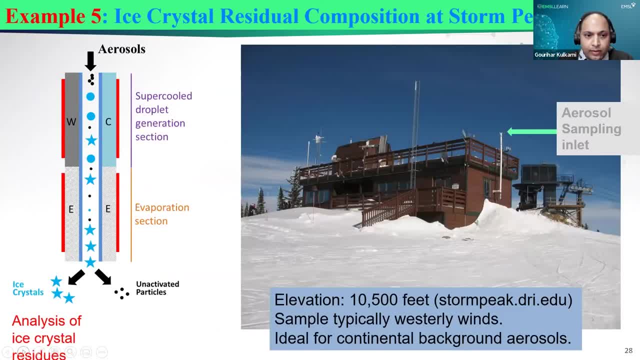 temperature dependency there. So that's the way this is going to be. In the past, the chamber has been deployed at the Stompec lab. The idea was to characterize the ion pay efficiency of the- you know, this continental background aerosol, as well as the analysis of ice crystal residues. what the composition of those 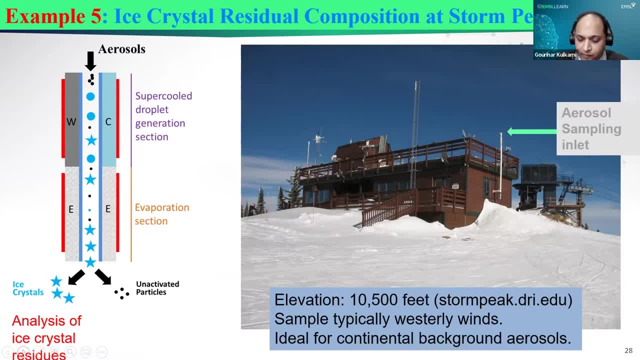 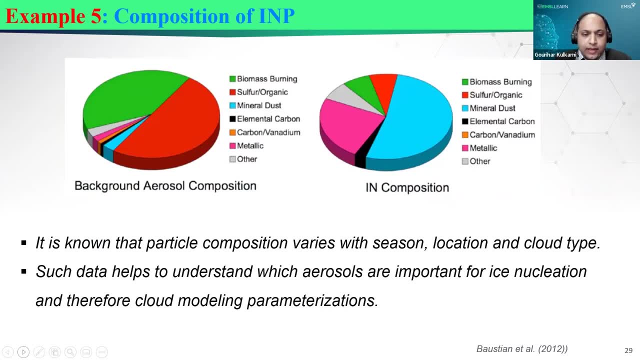 is. I'm not going to go over the results of ion efficiency, but I think it's important to highlight the composition results here, And you can see that there's a lot of residuals coming out of this chamber results here, So you can see that on the left is the composition of the total aerosols. 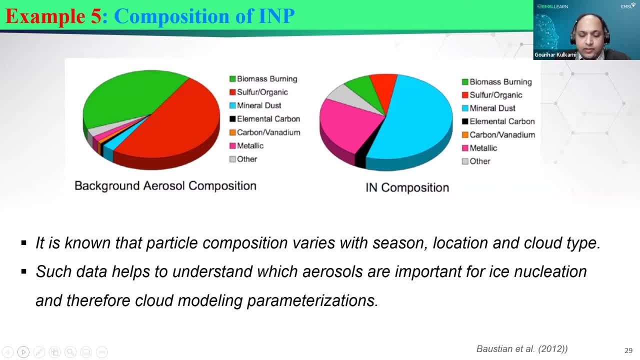 and on the right is the composition of the ice crystals residues or the INP composition, and you can see there's a difference there And such you know results are important. such mixing state data is so important to develop the INP panelizations which are actually needed. 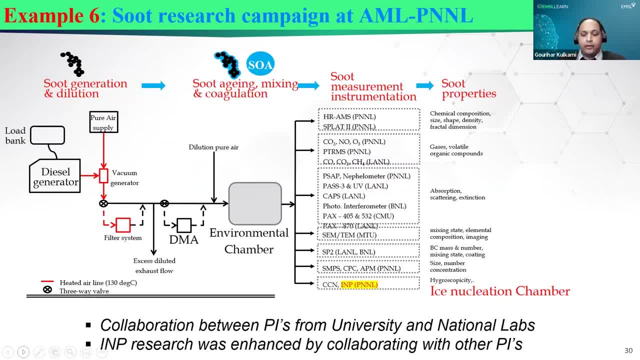 And finally, you can deploy the chamber as a part of a research campaign. So here is an example where the chamber was deployed with other co-located instruments that provided the composition provided, the gas phase properties, optical properties, mixing state properties, hygroscopicity, site distribution. And what you can do is you can. 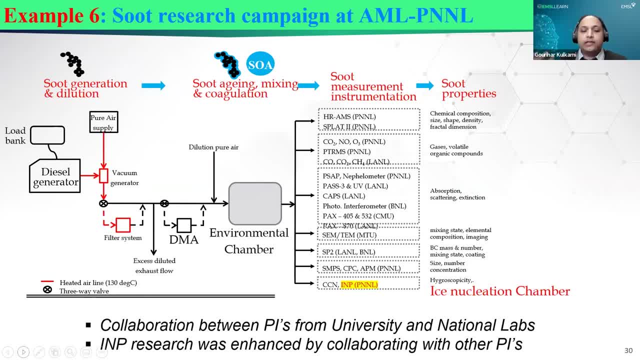 combine all this data set to understand more about the, the INP itself. That's what we're going to do here. We're going to go ahead and show you how to do that helps to understand or to develop the another parameterization for the model. 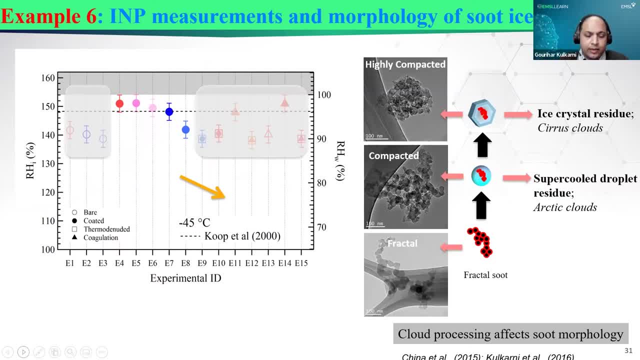 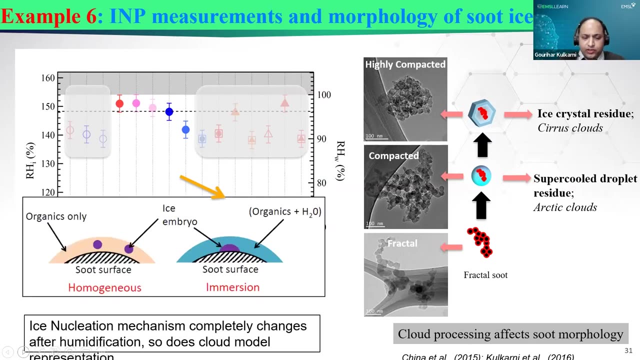 So here is example showing you the, the onsets at different experimental conditions and the temperature. showing you the, the, basically how experimental condition changes the onset. What you can further do with this information is you can develop some hypothesis of ice inflation mechanisms and that you can use that to develop the parameterization. 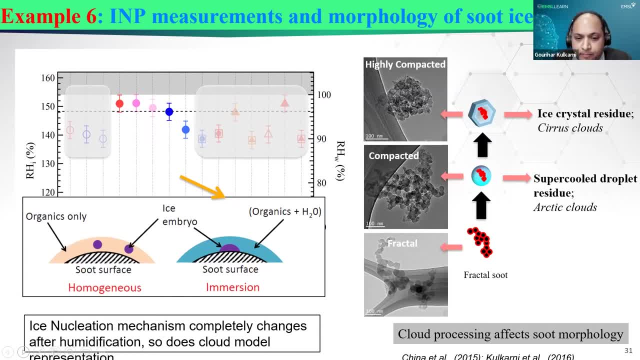 for a model. And finally, the figure on the right shows the you can look at the morphology of ice crystal residues, as well as the supercooled droplet residues, and you can understand how the cloud processing is affecting the morphology. And with that I'll end and thank you. I'll send it to. 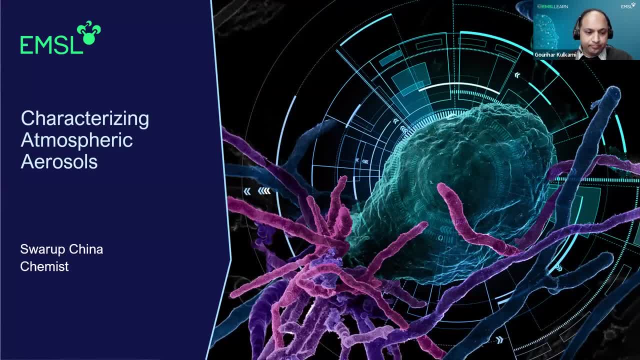 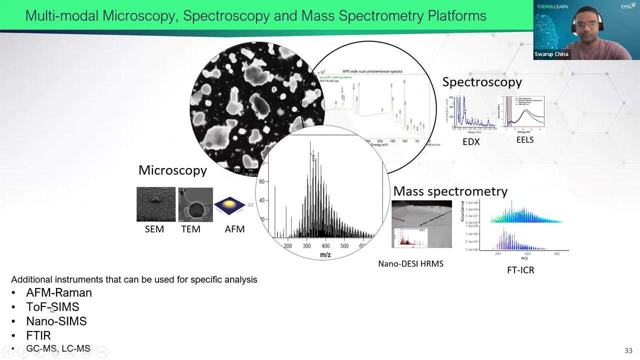 Swaroop now. Thank you, GK and Alla for setting up the stage, So I will briefly discuss about the different offline analysis method that we have at EMSA and how we can answer some research questions. Yes, so as Alla and GK mentioned, the atmospheric particles are often very complex and to try to 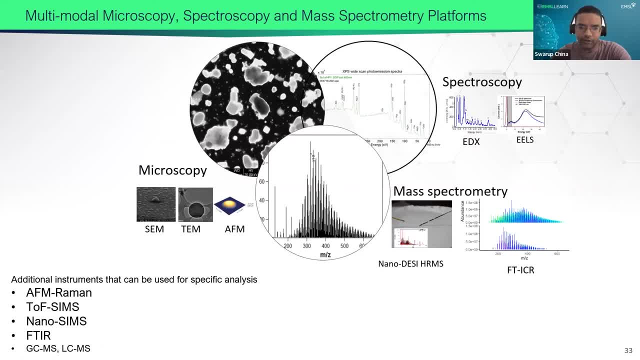 understand their different properties. we often look at different angles so we try to use multimodal approach, looking for microscopy, spectroscopy and mass spec approaches to answer the scientific questions that we're trying to answer, And today I'll briefly mention some of the key approaches that we use. 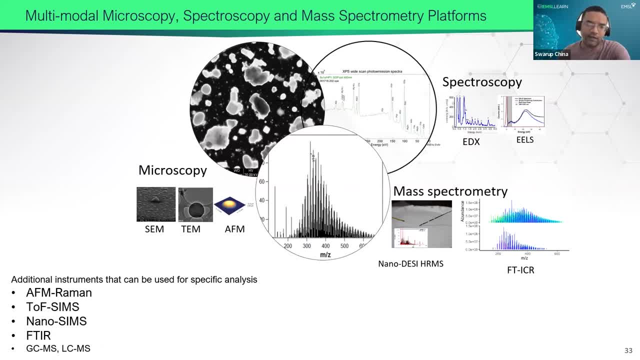 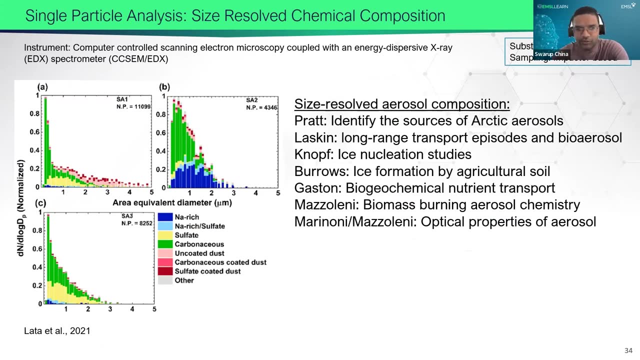 in our lab, and there are several others that are available at EMSA that I will not have a chance to explain in details, but if you have more questions, please feel free to ask. So one of the instrument that typically used to understand the atmospheric processes in 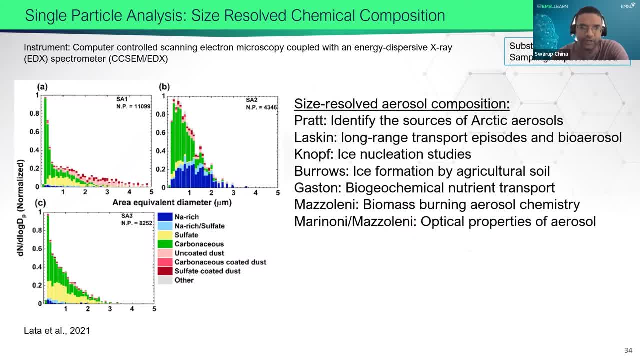 general is the size. result also composition, which is obtained by the computer controlled scanning electron microscopy coupled with energy dispersive spectrometer, the CCA-CMED-X. And in the east side, on the top right corner, I'll mention the substrate and the sampling approach that is used for different. 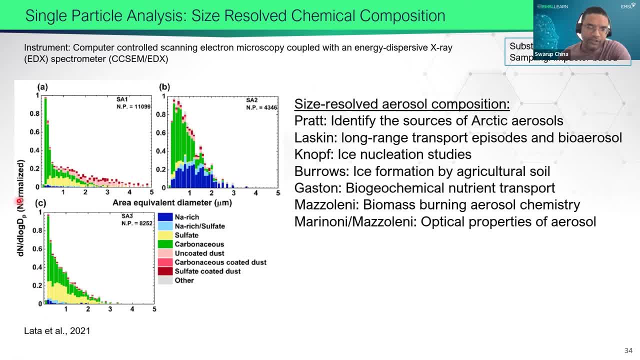 different methods that we apply. So on the left one you can see example. here is a size, result: chemical composition obtained from the CCA-CMED-X from a remote marine environment where we are trying to understand how different transport patterns affect the chemical composition. and here you get once you you look at individual particles and get the size and 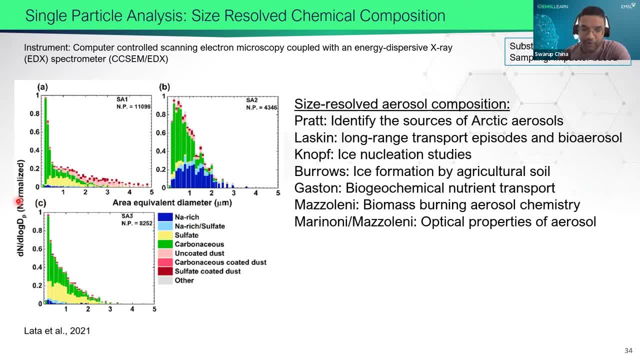 morphology and also the chemical composition- elemental composition specifically- and then you can classify the particles into different groups And this size result. chemical composition is a key information, as you see from ALAS and GK's talk that really needed to answer specific. you know some atmospheric science related portion and I on the right side, I highlighted some of the. 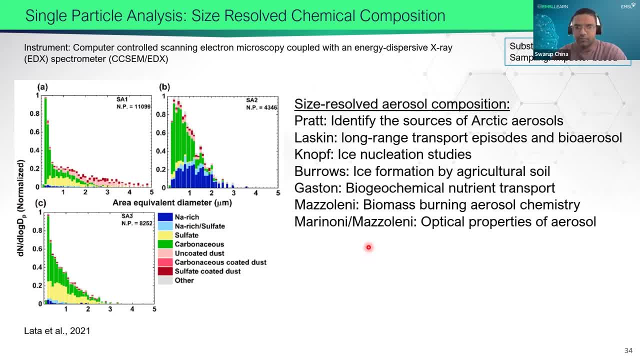 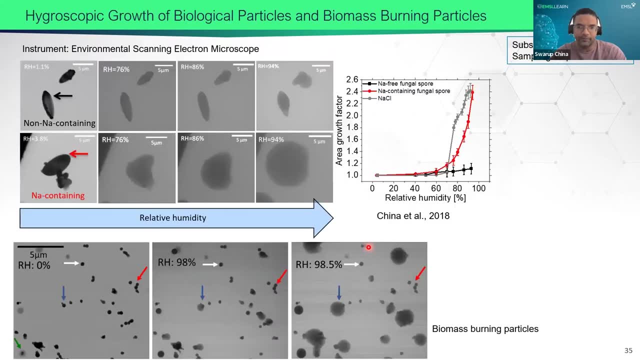 groups work that collaborate with EMSA regularly. kind of to answer different portions, like structure, the, where we want to look at the hygroscopicity of individual particles, and I just want to highlight that this is very key for when we look at the atmospheric particles. when you have a lot of light, 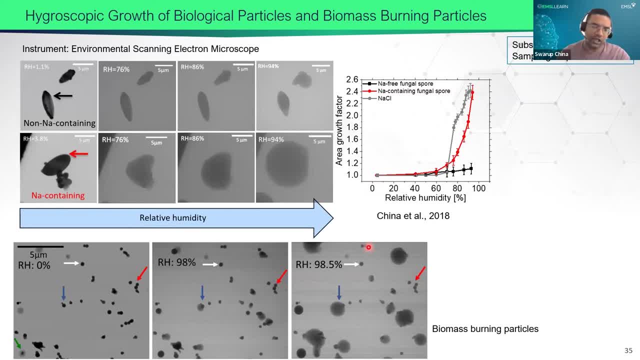 is in your particles. you expect a lot of different size and the composition. and here I'm showing one example on the top of biological particles and how, with controlled temperature and keep increasing the humidity, how you can see the growth of the particles and then you can see the growth factor. 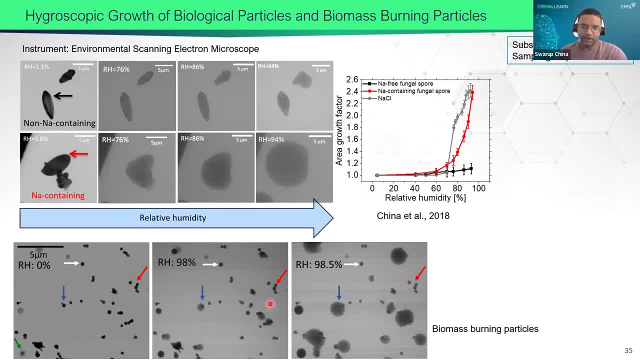 of the particles as a function of rate of humidity, And the below example is from the biomass learning also, where you can see some of the particles uptake water at 98.5- 98.5 humidity and others did not. So ideas that working out the Governor's discrete properties for the threechoic units. After the benefits of carbon Universally, we have been looking at how greenhouse materials change their body boundary twice in the course of class area technology wise, and how the present light and low tear pressure effectか find out the polymer that creates the power grid, or lock irgendwie, and topics like you. 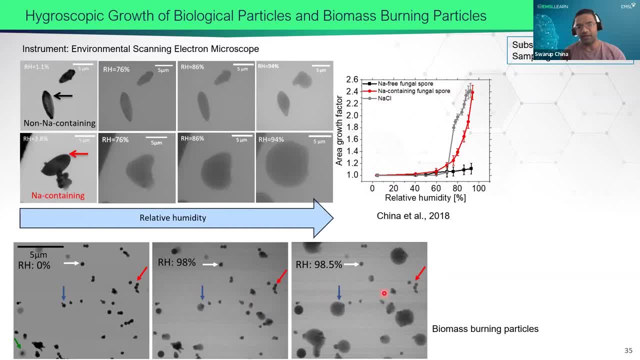 looking at the tracking individual particles and then map the elemental composition and the growth factor. then we can get an idea about how, which specific particles activated and which are not activated and what are the role of like size, composition and mixing state on the hygroscopicity of these particles. 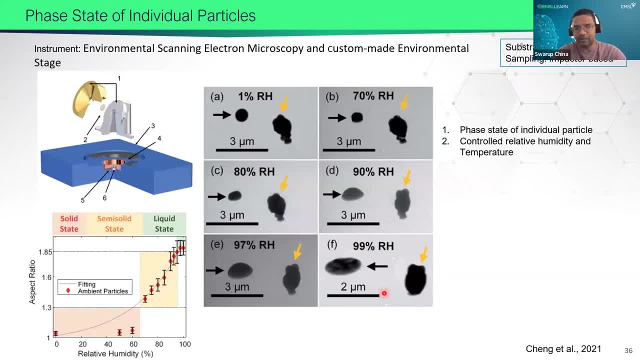 The next one again, I'll just again providing just a very brief highlight of different instrument that we have and how we can answer different scientific question here. So the next one I'm going to talk about is the same chamber, the same chamber that you use. 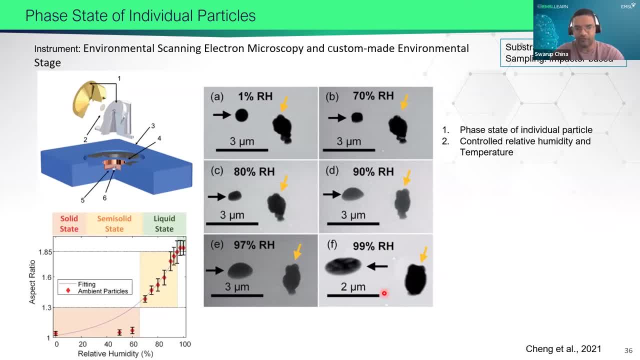 but it's a custom-built stage to understand the phase of the atmospheric aerosol which was explained by Ala and Jike. So these particles can be existing either solid, semi-solid or liquid state And we want to understand how this phase changes. 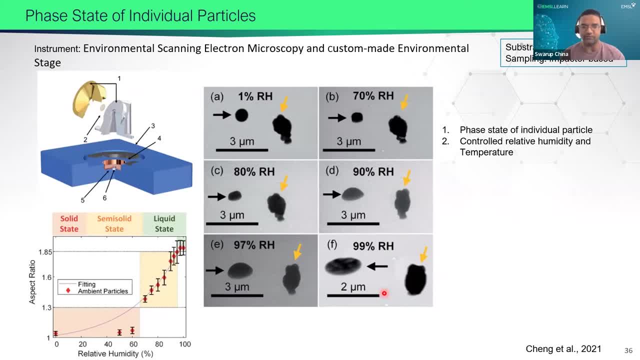 for atmospheric particles, especially at the submicron scale, as function of temperature and humidity. So with this stage we can look at track individual particles and we keep the temperature constant and then increase the humidity and see how the particles are changing the shape. 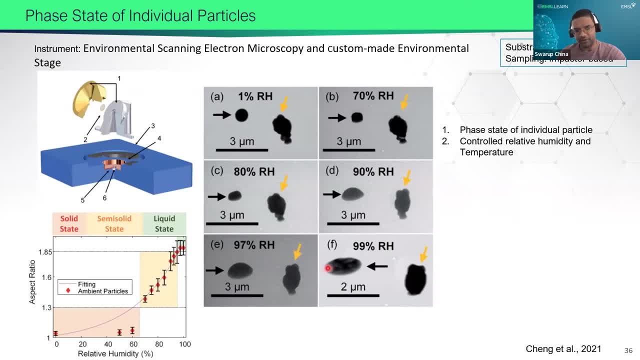 And you can see from looking at the tilt angle, as a function of humidity, it's the particles getting flattened out, So particles transitioning from solid to semi-solid and becoming liquid at the end. So again, this technique will be useful for when you are looking at specific particles. 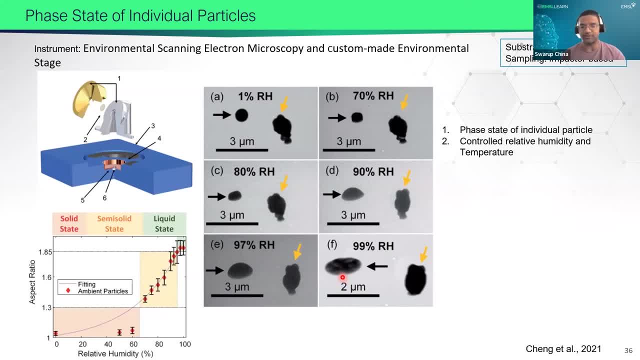 when they are submicron in size range and especially when the particle concentration is very low. So often we cannot apply the online instruments. We can collect particles on a substrate and then look at the individual particle phase state as a function of humidity. 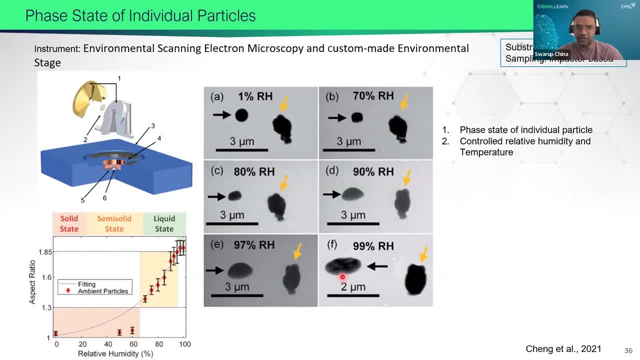 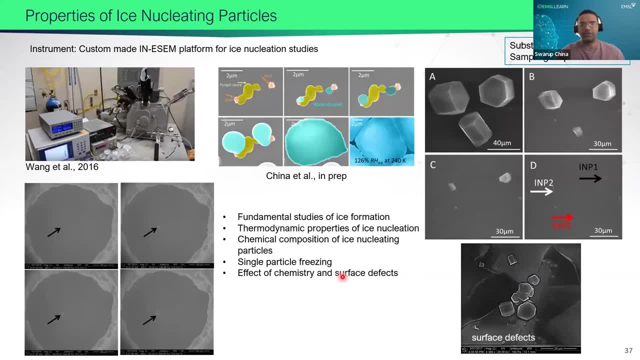 And for the temperature. we so far we can control the temperature to minus 10 degrees Celsius for this kind of experiments. The next I'll mention about the ice formation again, which was mentioned before, And this is a little bit defined approach, what GK mentioned. 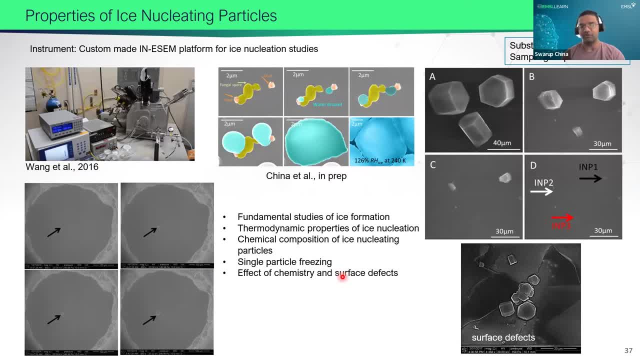 where, instead of getting higher statistics and frozen fraction, here we are looking at more like a fundamentalized formation- And I'll explain briefly- like how these defined experiment are set up. using the same instrument can give you a specific portion that you can ask. So here you're looking at the opening of the scanning area. 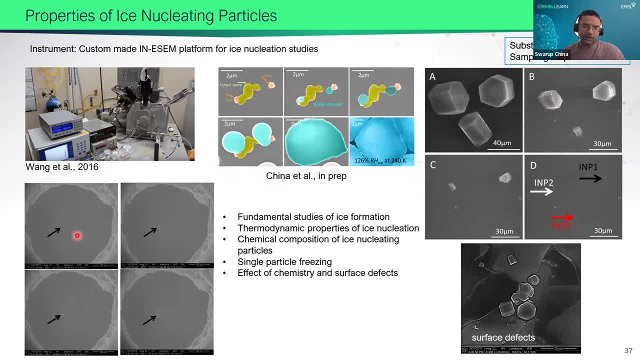 that we're looking around 500 micron. This is the aperture of the electron gun in the ESEM mode, And then you can keep decreasing the temperature of the substrate and basically increasing the rate of humidity with respect to ice, And you can see from where ice is start forming. 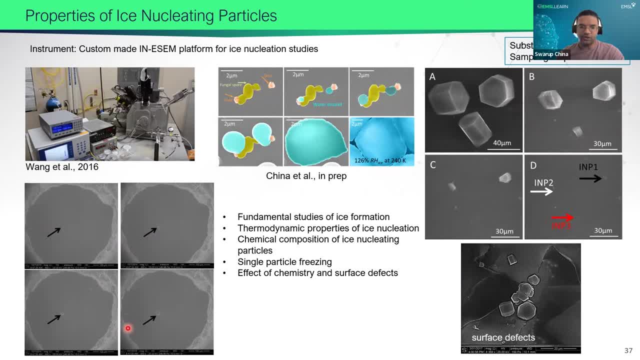 And then you can get the thermodynamic properties like temperature and the humidity where the ice formation started. Other case: if you really want to focus on single particle fizzing events like you really want to understand, like if you have an internally mixed particles- 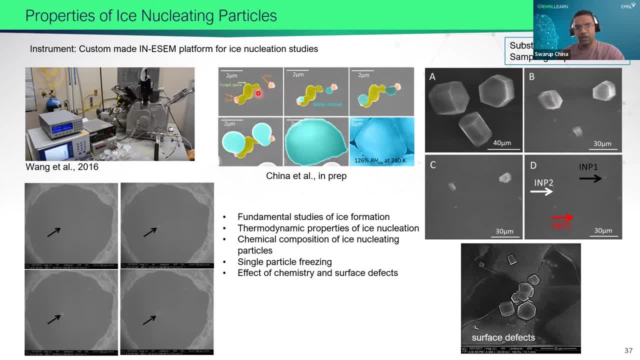 then from where the ice formation started. so we can zoom in into one of the individual particles and try to see from where the ice formation started. And this is one example in the immersion mode, where you can see the dust particles mixed with the biological particle. 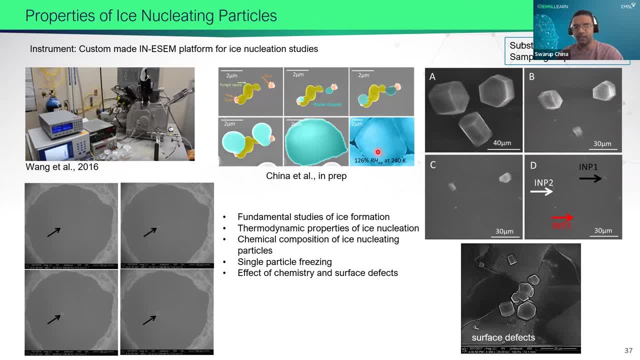 is start up taking water and then finally form the ice. Other thing, what GK was mentioning about the INP residuals. So here again, instead of looking at the separating the residuals, what we do is we form the ice and then we start sublimating the ice. 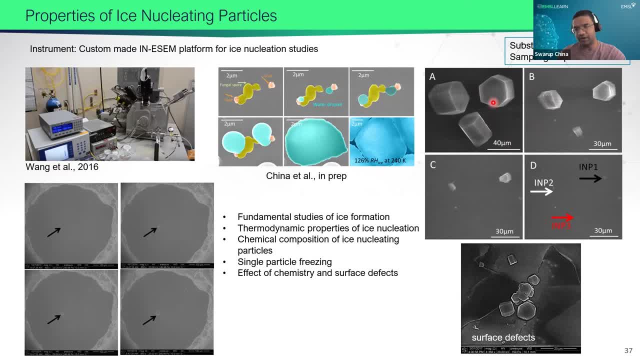 So you can see, for example here there was a three ice crystal form on the substrate and then we start sublimating the ice And then we can track those individual particles and try to get their size and the composition and see what are the specialty about those particles. 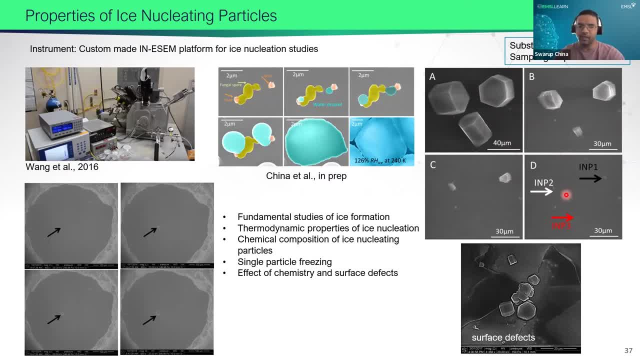 and then compare with the total particle population. And the other experiment that you can design is that looking at more surface defects, So you can motivate your substrate, changing the composition of the substrate, and then get some surface defects And you can see at high specific resolution. 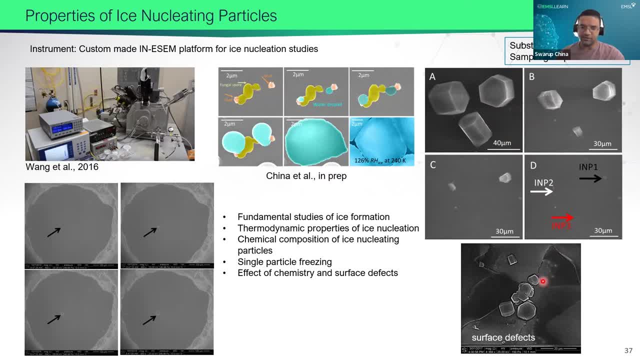 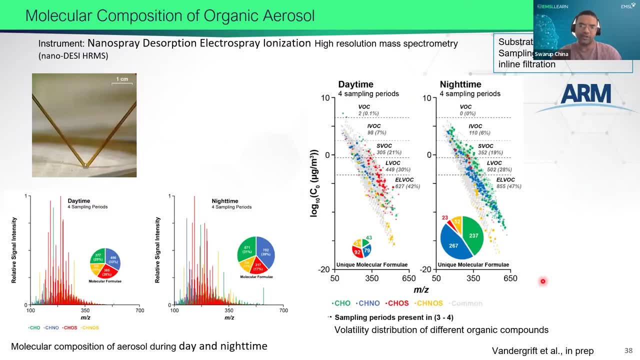 that from where the ice formation started. This is example from a natural micro substrate. Next I'll move to our high resolution mass spec capability, And at EMSO there are like defined mass spec capability are available, So I'm talking about the one most we that we use. 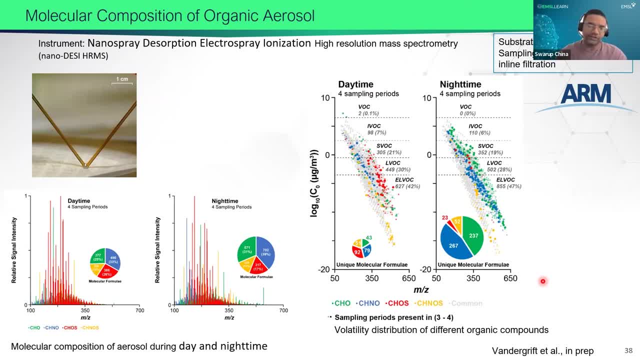 for our services that we have in our lab. It's a nano DC high resolution mass spec And this can be integrated into any mass analyzer, is an orbit web or FDIC. So this is a very high resolution mass spec capability that we can use for our instruments. 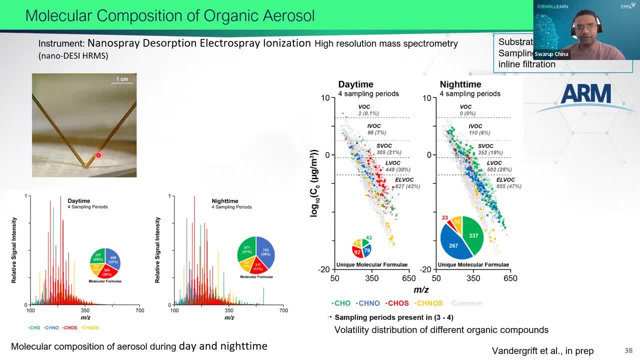 So for nano DC the advantage is that we can look at the molecule composition directly from the filter, especially for our source samples when the sample mass is quite low, And then we can look at the molecular composition. Here I'm showing one example. 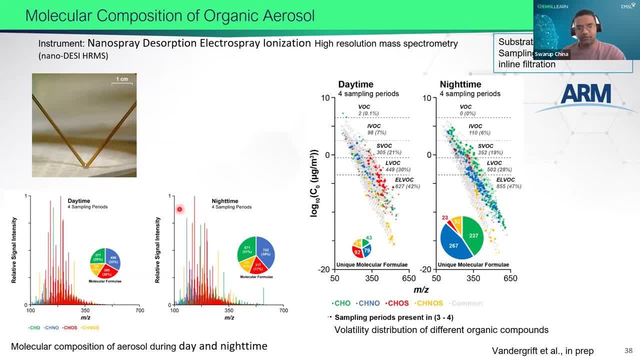 of looking at the organic also composition and at the one agriculture land from DOE arms site where we're looking at the how the molecule composition changes during daytime and nighttime And the light panel shows the productivity distribution that I was mentioning. that is really critical to understand. 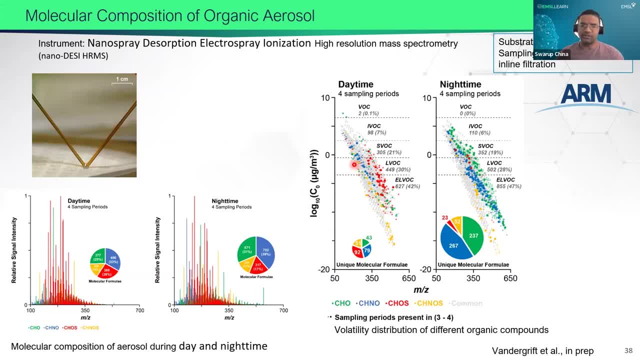 and the growth or the evaporation of the particles. We really see the dynamics, how the particles, they are involved in the atmosphere and at the molecular level. So next, I was talking about so far the physical and chemical properties, And now I'll move to the optical properties. 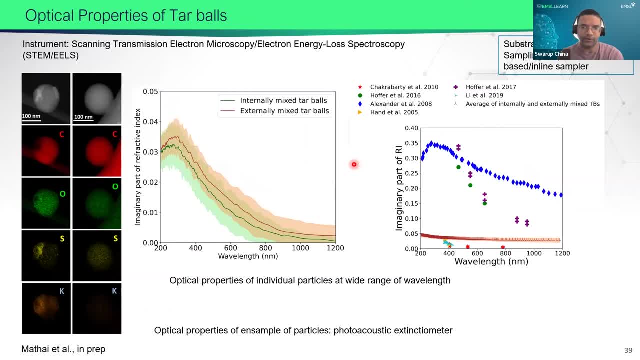 So I'll briefly explain. one of the capabilities that we have is scanning transmission electron microscopy with electron energy loss spectroscopy And with this technique you can estimate the optical properties of individual particles and the board wavelength region. So again, the idea is that when we really try to understand, 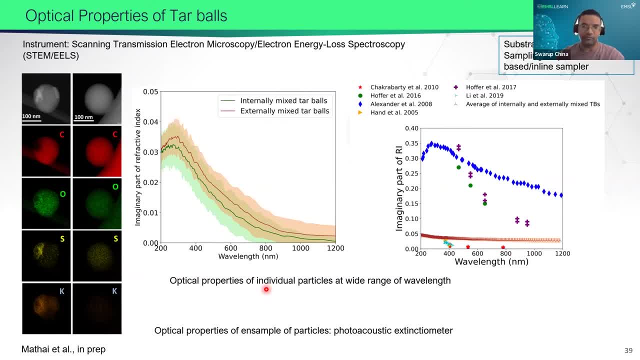 the optical properties of in the atmosphere. there are a lot of different mixture of particles And if we really try to understand one specific, specific class of particles, then we can look particles one by particle-specific optical properties. The limitation of this method is that you 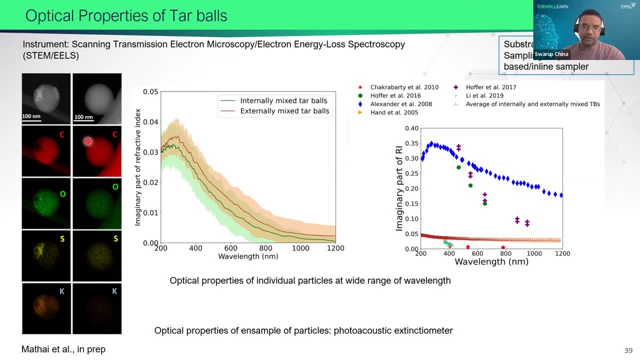 can do only for particles that are spherical in shape, a particular size range and also need to be resistant to the electron beam. So here I'm showing one example of one specific type of particles that are emitted in the smoldering phase of the fire. 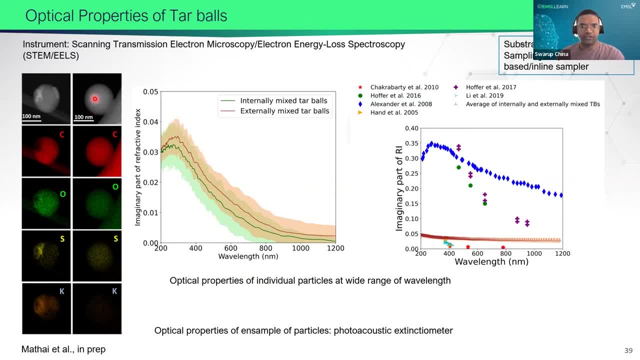 And here we're looking at both. one example is more like homogeneous mixing- One is internally mixed particle- and try to see how the effective index changes And then from that we can derive the optical properties. And the advantage is that here we can look at the wide range. 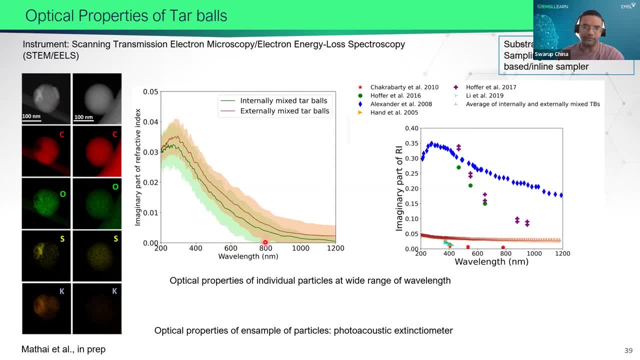 of wavelength, which can be really useful for climate modeling perspective. Other method: we have also the photoacoustic extinction meter where we can look at and some of our particles is trouble can individual particles, And that can be. that is in-situ instrument. 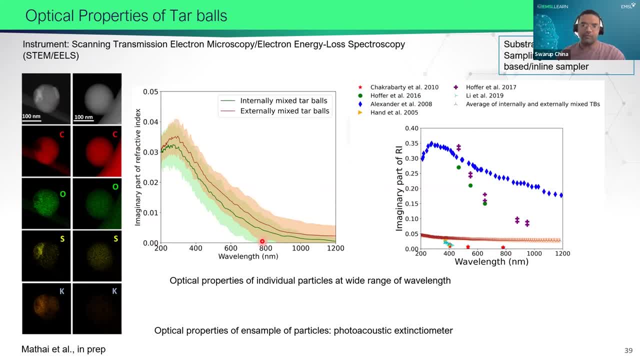 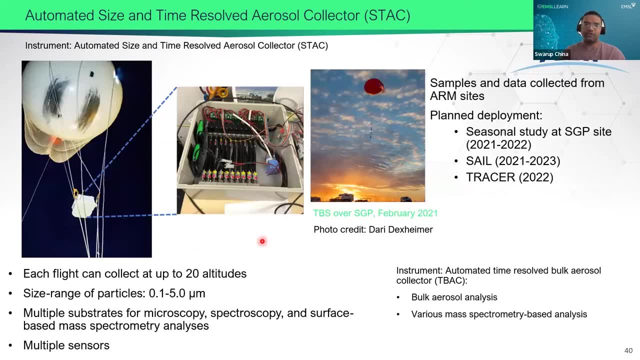 where we can look either lab-generated aerosol or the ambient aerosol samples. The next I'll briefly mention about recent collaboration And I know that some of you asked specific question about this topic And, as you see, also there was a call came out from the ARM. 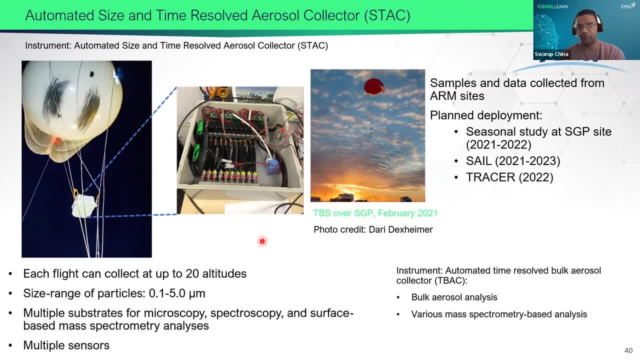 and EMSO FICUS project. So this related to one project that is in collaboration with ARM And we developed a size and time result aerosol collector for arms sampling, And so I guess that we really want to look at the particle profile of aerosol composition. 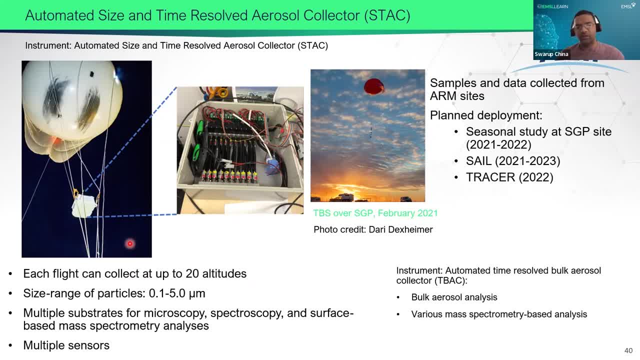 to answer a specific question, either related to land-atmosphere interaction or, if you're looking at the aerosol cloud interaction. So we built, in collaboration with ARM, an impactor which can be fitted with a TBS system. This is relatively small in size and high collection efficiency. 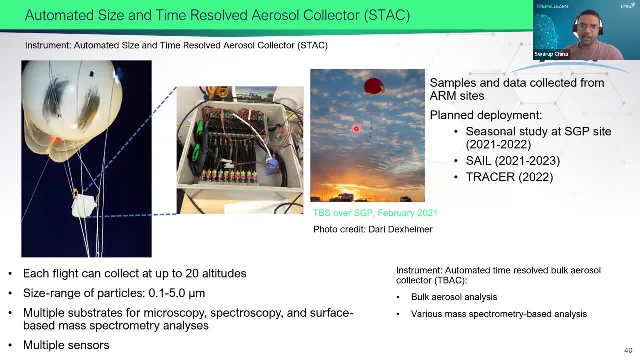 And that can go at different altitude And looking at the different layer in the atmosphere and see how the composition and the size changes. And there are multiple substrate of this look arranged on this impactor So we can do all different kind of analysis that was mentioned in my previous slides. 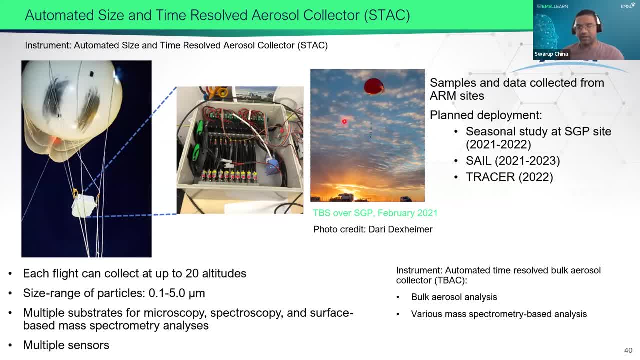 And so far this has been deployed in Alaska and at the SDP site in Oklahoma and also some initial flight testing at the SAIL campaign And the stack will be deployed with the TBS system in the upcoming campaign starting from next month, actually at the SDP site. 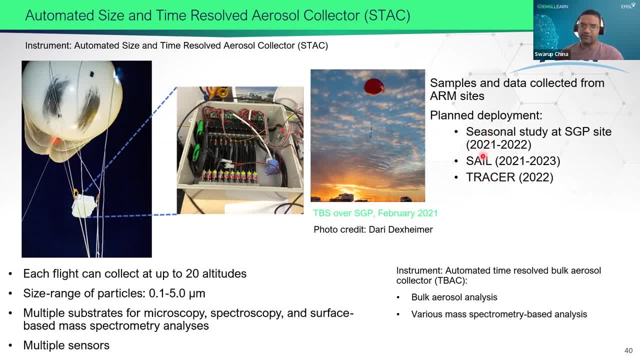 we'll do the seasonal study And also it will be deployed at the SAIL and TESOL campaign And in addition, there was a limitation of amount of particles that we deposit for the stack, because this is specifically designed for single particle analysis. 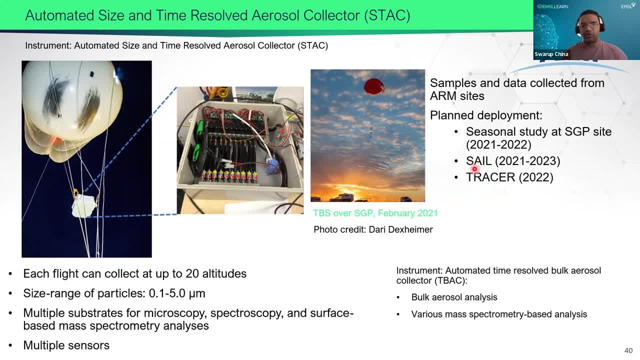 So, as you expect that we often don't get enough mass for high resolution mass spec analysis, We performed some analysis when the concentration was very, very high, But often if you have a particle concentration of 500 particle per cc, it is difficult to get enough particles. 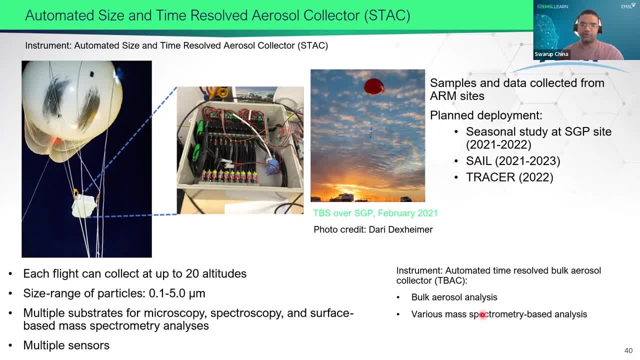 on the substrate. So for that we also planning to deploy a time-resolved bulk evasor collector which will collect the bulk evasor, which should give a sufficient amount of particles for a defined kind of bulk analysis method and also have extraction-based high resolution mass spec. 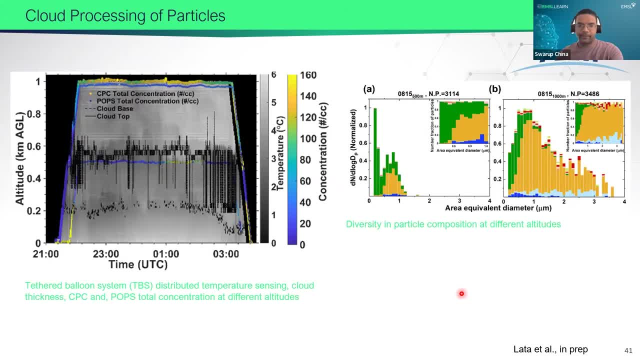 analysis. I want to show one example of the activities with the ARM campaign. Here you can look at one example from the Alaska site in the We're looking at the different layer of the clouds And the good part is that also we have some instrument from the ARM site that 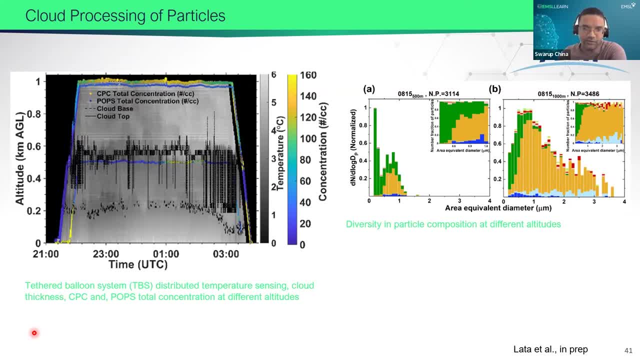 can be used for both evasor and cloud properties in conjunction with the DPS system. So here you can see an example that we're looking at the above clouds and how the size and the composition changes. as we expect, You see a lot of sulfur particles at the above clouds. 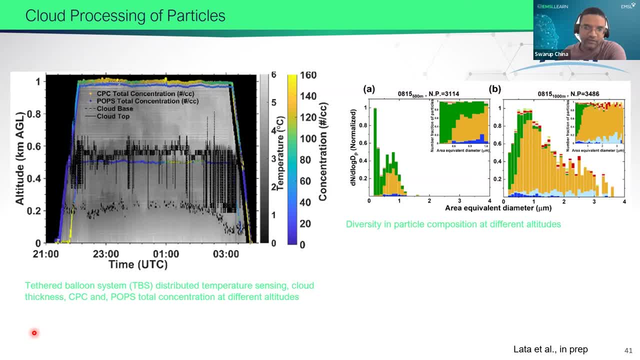 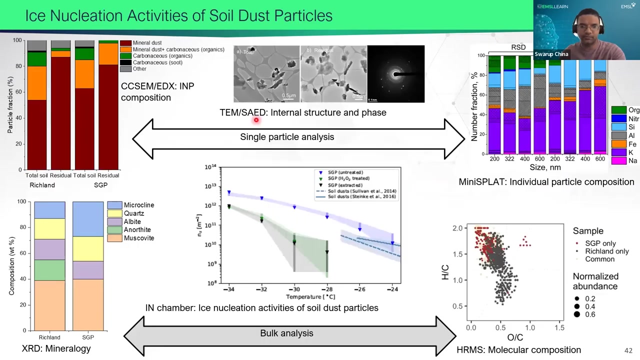 And then you see a lot of carbonaceous and sulfur particles in the clouds. So you can really look at the different atmospheric processes that are happening in cloud or above cloud and try to understand of these properties. Next slide: So I'll end up with this slide, which 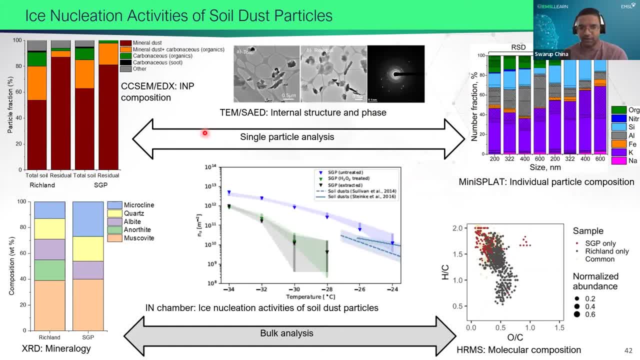 was kind of a summary of some of the methods that are already explained by Alaa and GK and our offline analysis. So we are trying to understand the ice nucleation properties of a soil dust particle. So this is done using GK's ice nucleation. 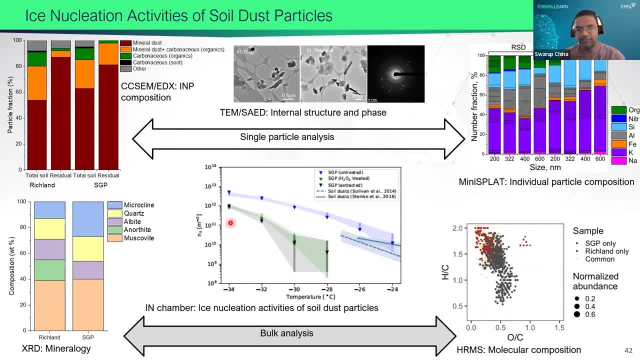 chamber and trying to define the soil dust particles and try to understand why the difference is ice nucleation properties. So we applied as our single particle approach, using both CCS-CMEDx and also Alaa's SPLAT instrument to try to understand what are the difference between these two. 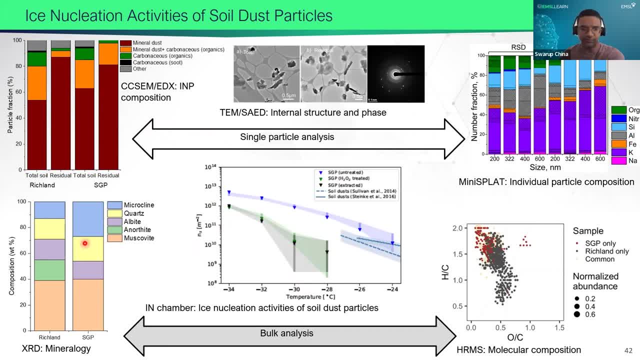 soil, dust, And then also looking at the bulk properties, for example using the X-ray deflection method, looking at the mineralogy of the dust, the dust particles, and then extractors for organic matter, because we observed a difference in ice nucleation properties. 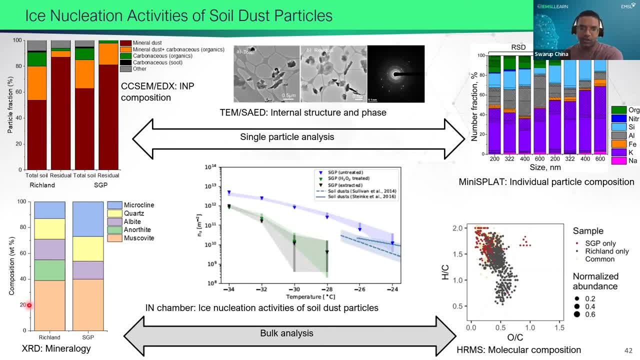 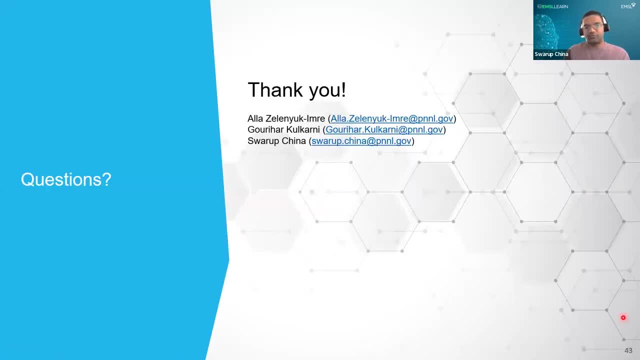 of these extractors for organic matter and try to understand if we can explain at the molecular level the ice nucleation properties of these particular soil types. With that I will finish, And please feel free to ask any questions, And I also leave our contact information. 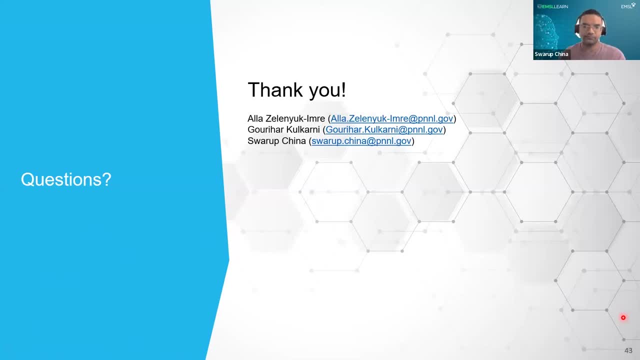 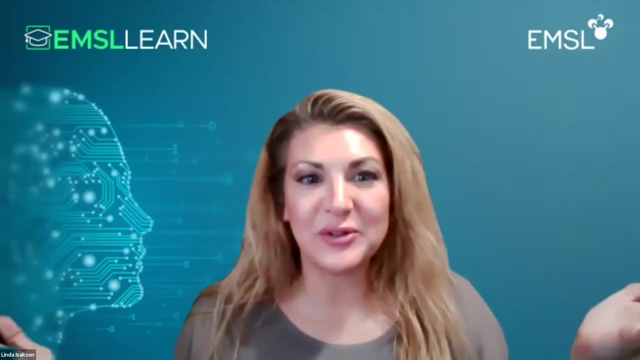 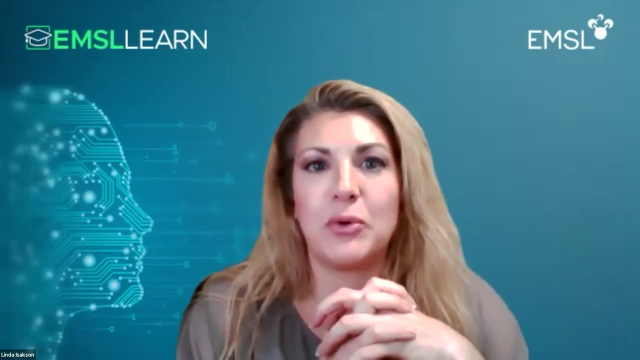 if you have any specific questions for us. Thank you, Excellent. Well, thank you everyone for your amazing presentations. We are now moving into the Q&A portion of the webinar. So again, folks out there, if you have questions. 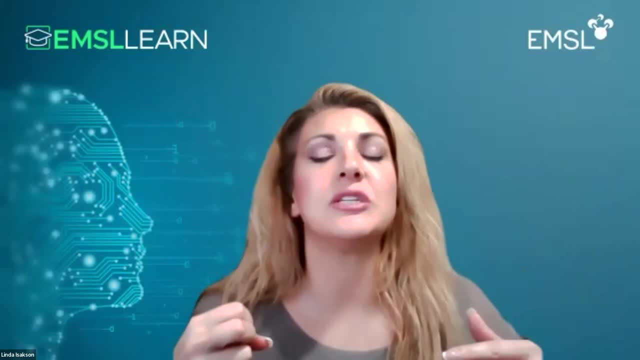 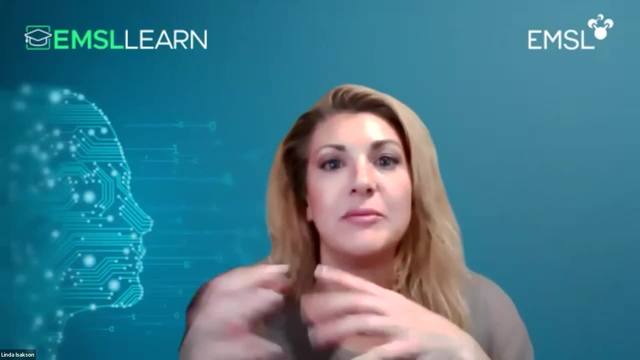 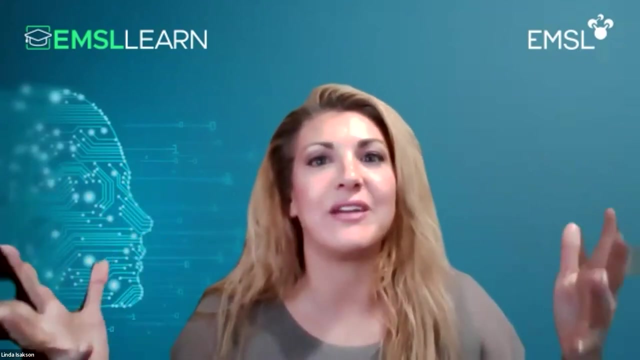 make sure to drop them in the chat. We've been pulling your questions that you've asked during the presentations, And so we're going to start talking about them now, And if it inspires more questions, other people's questions again, feel free. 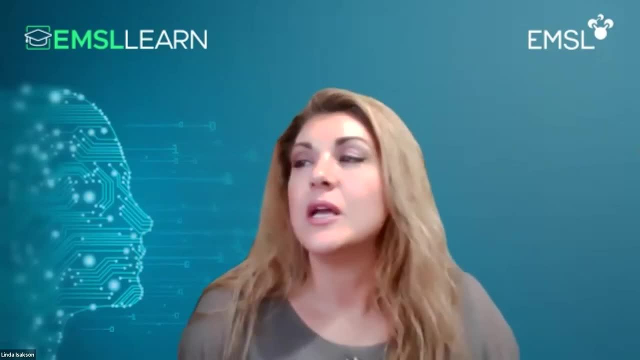 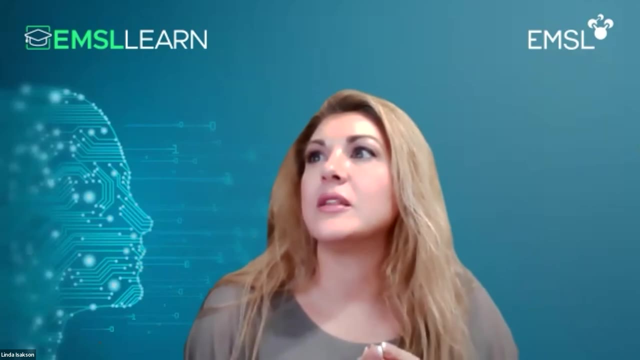 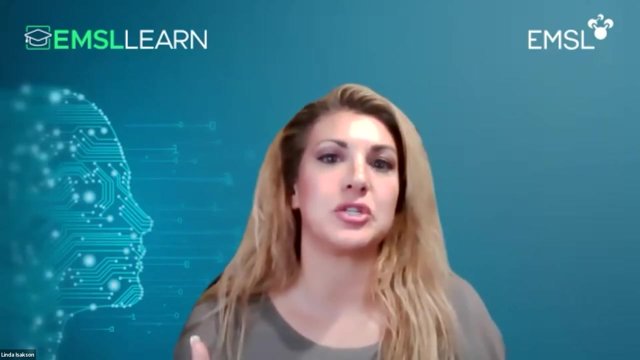 drop them in the chat and we'll get to them. So to start, let's see. So, Ala, we had a couple of questions for you. Let's start with what makes EMSL's aerosol mass spectrometer different than other similar instruments. 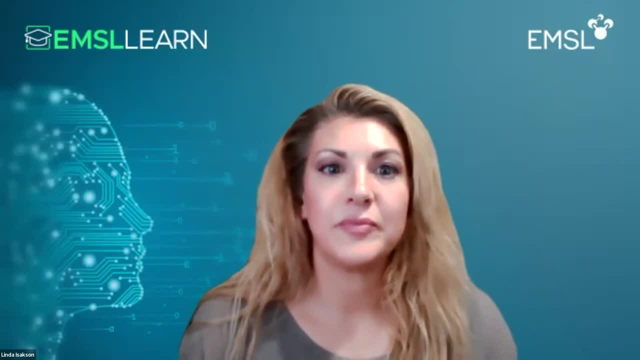 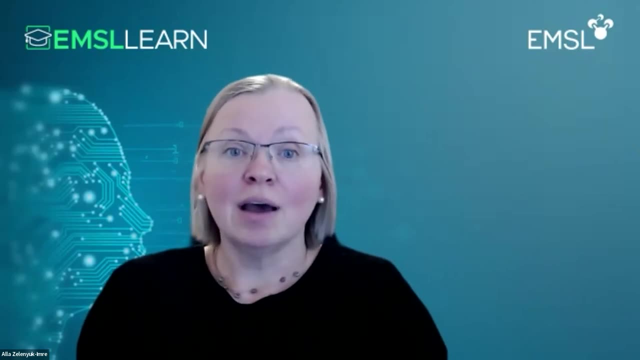 in the field. ALA TORRES- Well, I think first of all, it's a good question. First of all, I would like to point out the difference between the mostly common use aerosol mass spectrometer AMS, Unlike AMS, which looks mainly at bulk aerosol composition. 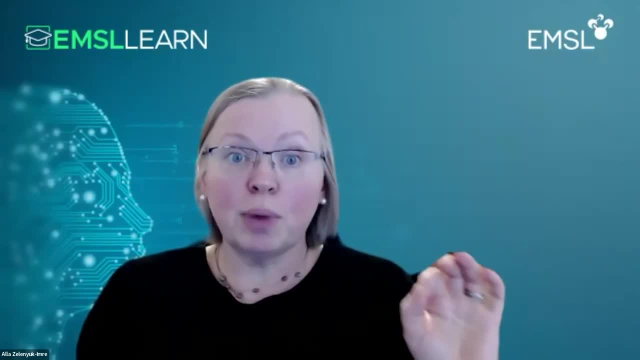 of non-refractory. SPLAT looks at individual particles, both refractory and non-refractory, in each individual particle, So it is a single particle mass spectrometer. Compared to other single particle mass spectrometer, I think we have significant differences. 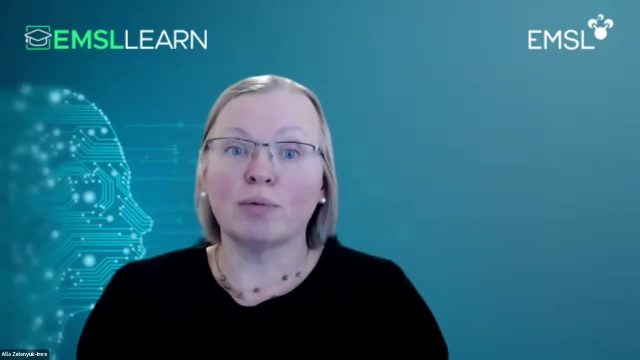 We have significantly higher sensitivity, especially towards small particles. Often, I said, we have our mantra: If there is one particle PCC, we could detect it in one second, which enables many of very unique studies And, moreover, this multidimensional analysis. 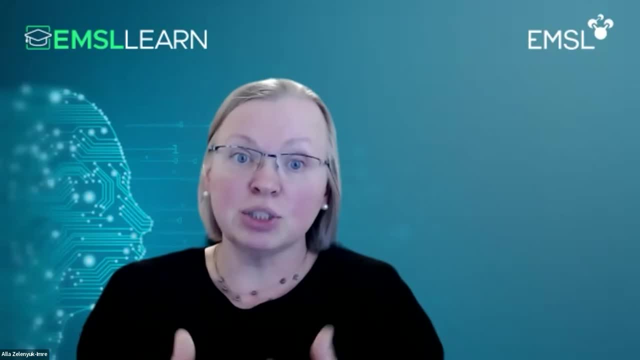 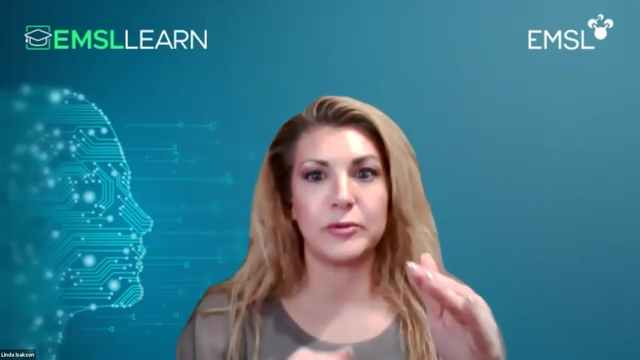 where we're measuring many different properties from the same particle is something which makes our instrument not very special and allow us to learn a lot, but also makes it quantitative. OK, We have a couple more questions for you, Ala, but I'm going to rotate through. 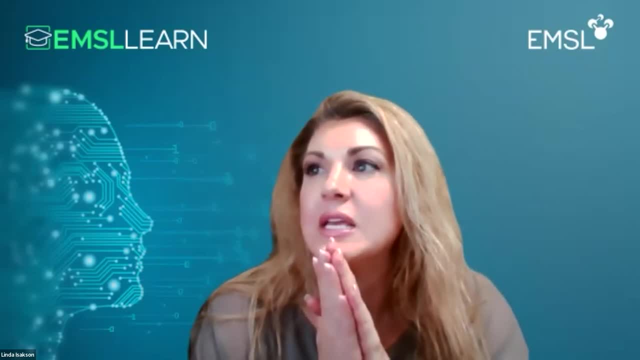 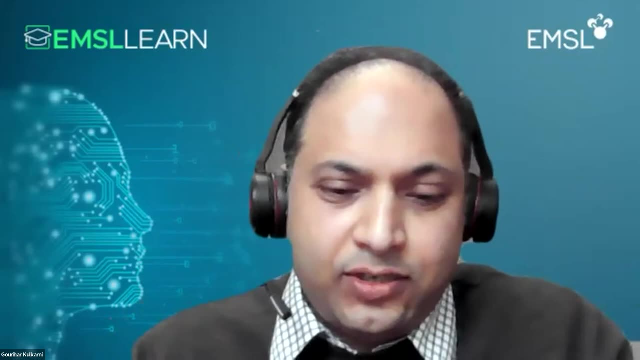 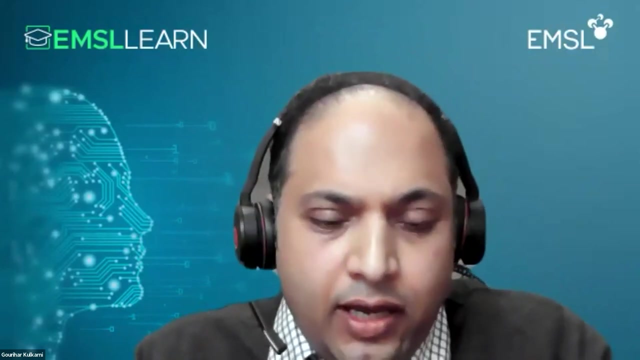 So, GK, we've got one for you. Can the ice chamber be deployed in the field? That's a good question. So ice chamber has the capability to deploy in the field. You can run that in autonomous mode also And you can scan at different temperature, and it could be. 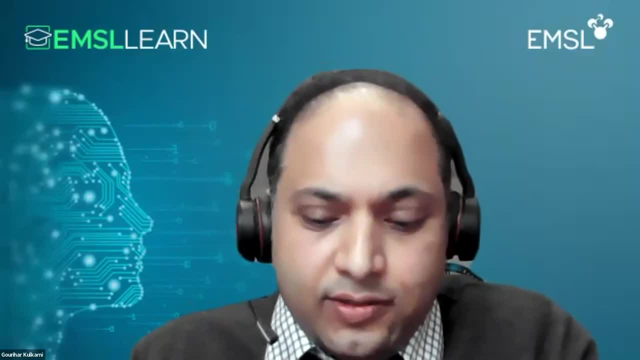 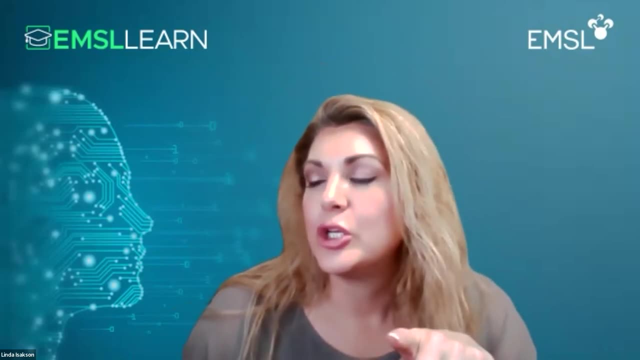 part of it. It could be part of any other co-located measurements too. So yes, answer is Yeah, all right, And then one for you. Shorup, You referred to the IN-ESCM method, but the resource needs template refers. 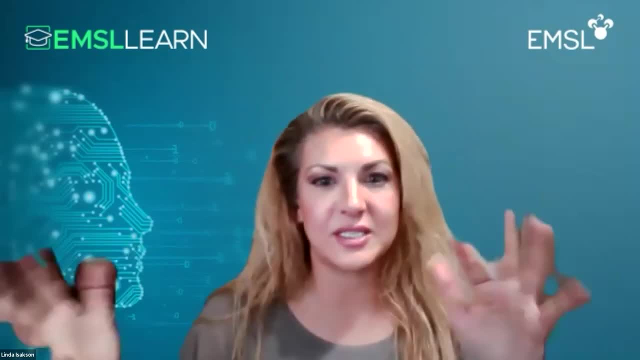 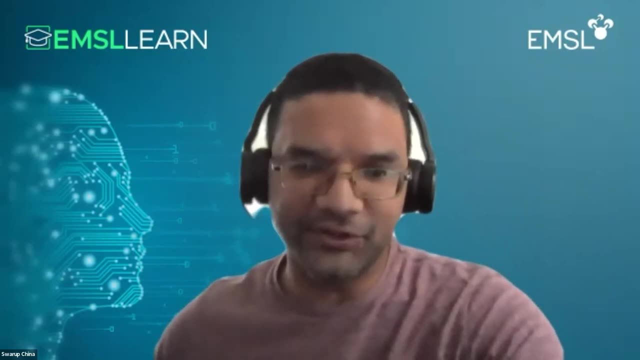 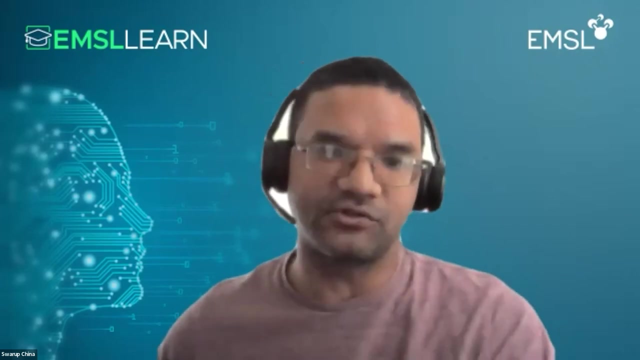 to environmental transmission electron microscopy. Is this the same? No, it's not the same actually. So, Yeah, sometimes it can be misleading. So the instrument that comes under this is called computer-controlled scanning electron microscopy. then slash high-speed equation stage. 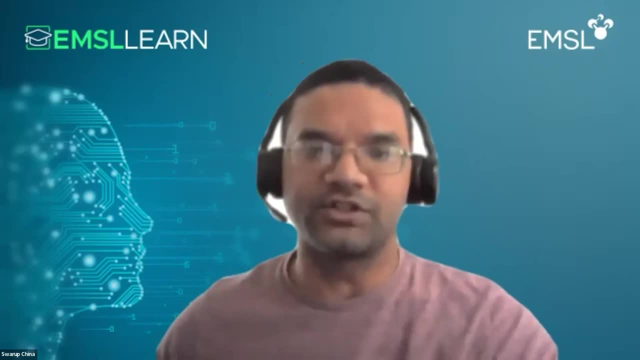 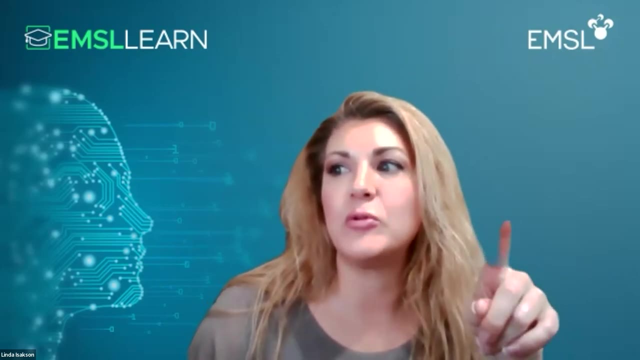 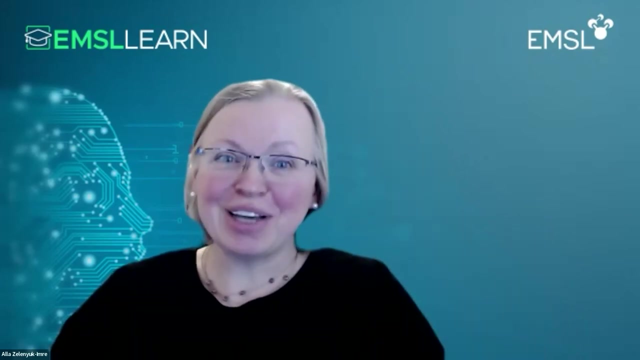 So that's the instrument that is listed under the ISO characterization. All right, Ala, back to you. Has MiniSplat flown on, or can it fly on board ARM's tethered balloon system? No, it cannot. It could fly on aircraft. 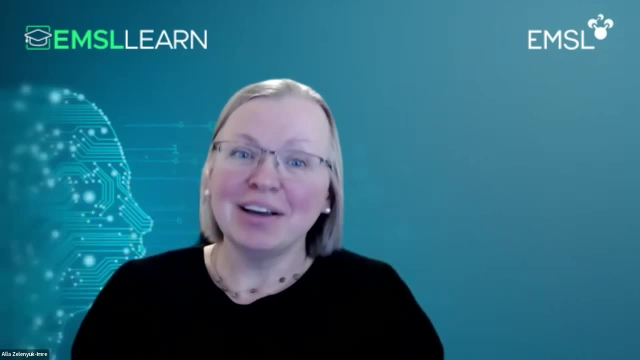 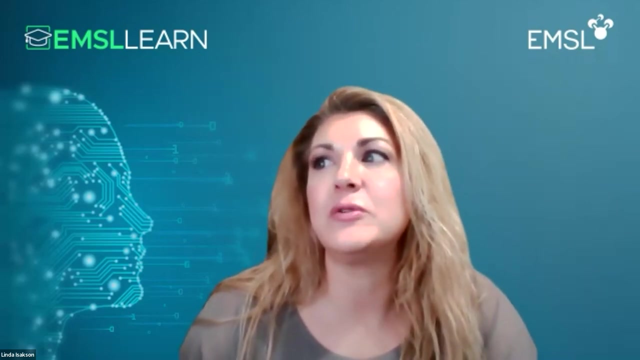 But it cannot. I mean, it's not yay big, It's not handheld. So we do our measurements, altitude-dependent measurements on board of aircraft. OK, And GK back to you. Would you train users to operate the ice chamber? 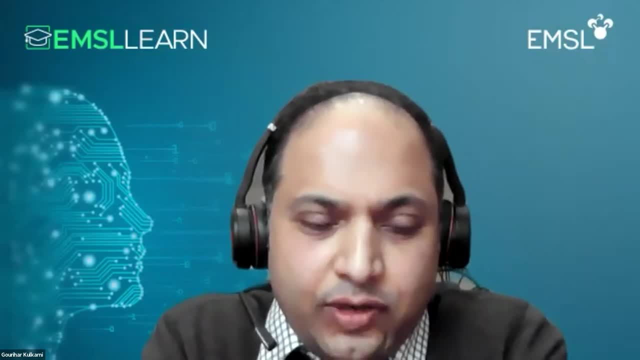 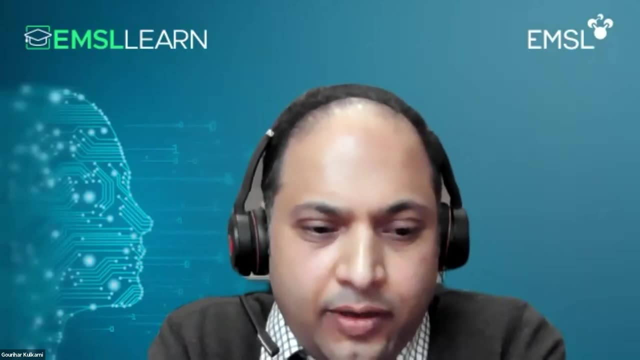 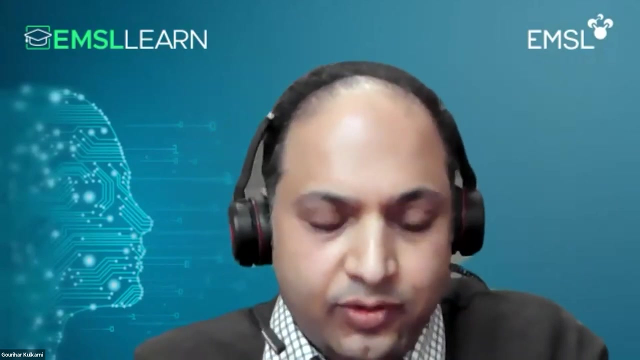 Yes, I do So. it's like a half day to two days training. any user can really use it either in the field or in the lab. All the software operations are fully automated And it's very easy to do those operations OK. 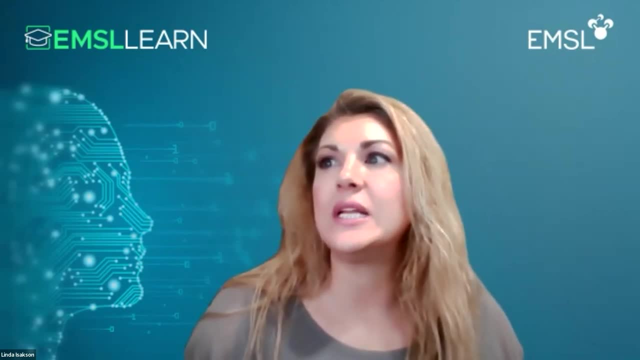 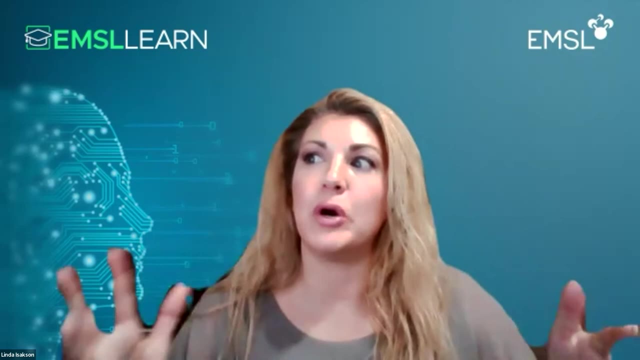 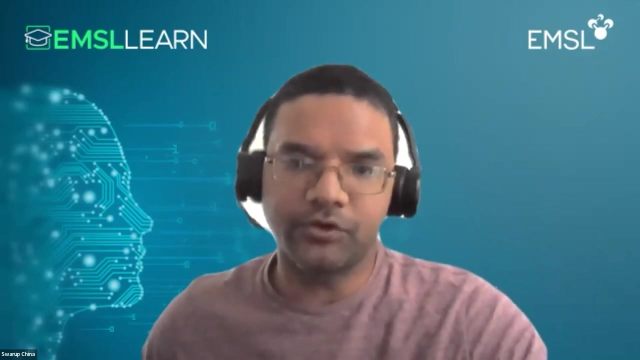 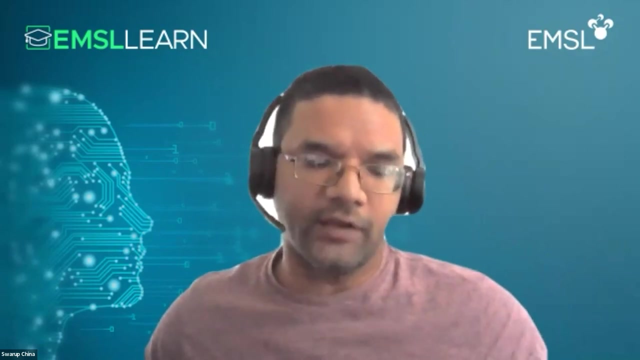 Swaroop, let's see What is the temperature range that single-particle freezing experiments can be performed. Can you do both deposition and immersion freezing experiments? Yes, The chamber can do both deposition and immersion freezing experiment And typically we use for between 205 Kelvin to up to like 255,. 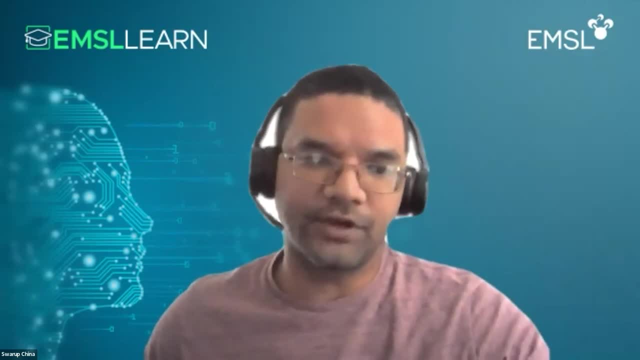 260 Kelvin, But if you look for single-particle freezing events, typically the polar temperature is better. because you have this, We can clearly see the growth of the individual ice crystals. OK, And another question actually for you again, Swaroop. 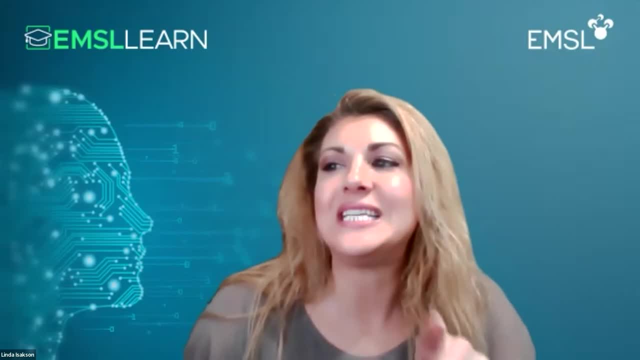 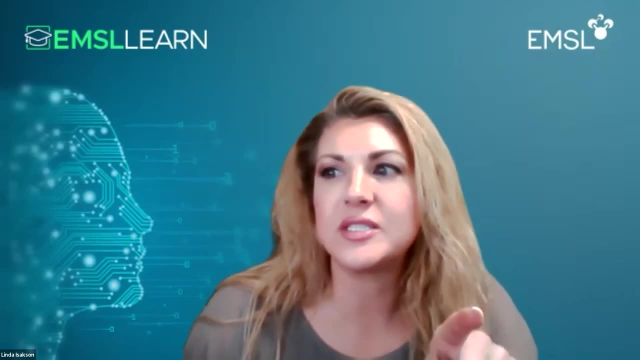 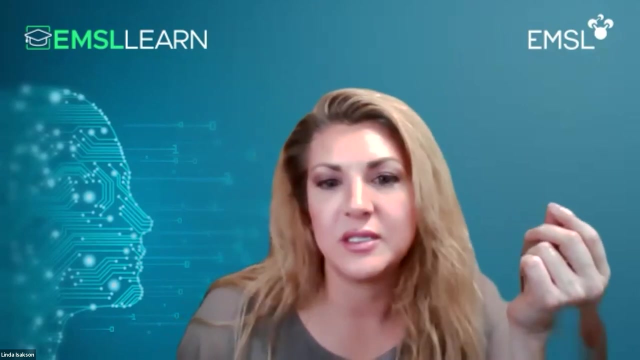 The SCM-D or EDS? what is the particle size range for measurements? Also, are thin sections necessary Or can you analyze raw samples, such as small quantities of dust particulates? So to answer your question, the SCM-EDX. typically. we. 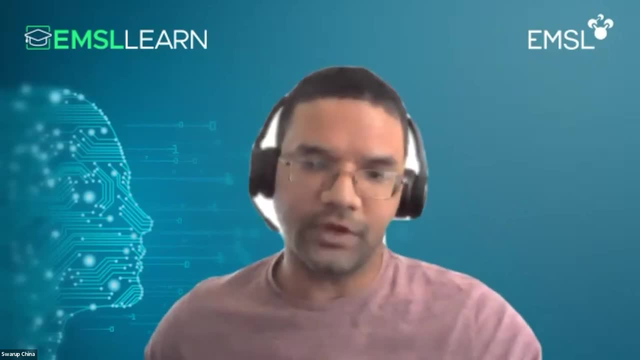 measure the size range from 100 nanometer to up to 5 micron, But it can be measured larger particles as well. Just So we need to make sure that when the particles are thick- that's related to the second question- If the particles are thick, you're. 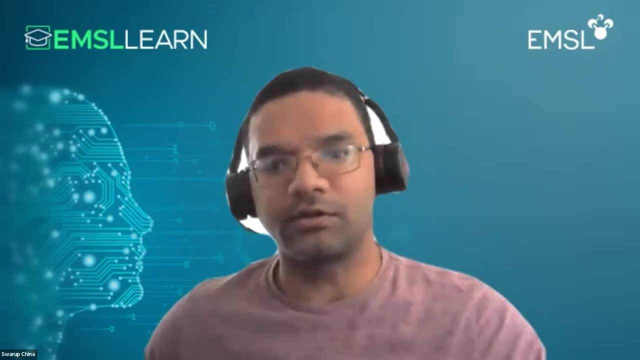 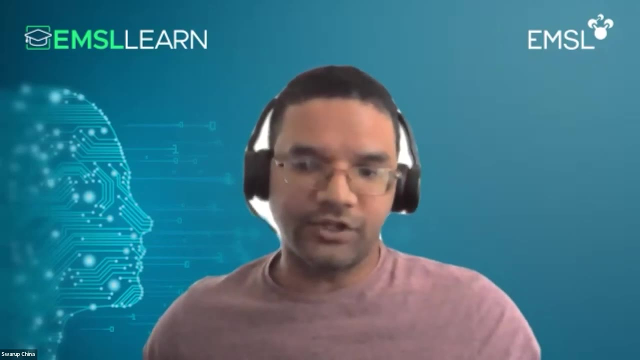 getting the composition from the surface. that depends on the voltage and the current you are using, Typically like around 1 micron depth of your samples And for our analysis we don't quote any samples. So that's the main advantage of using ESM. 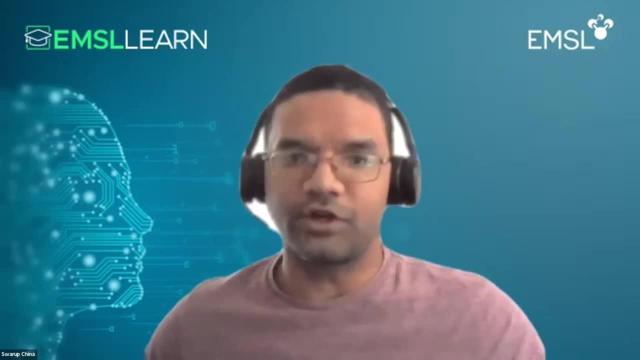 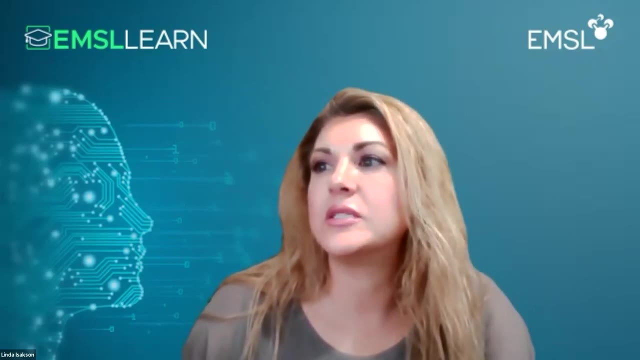 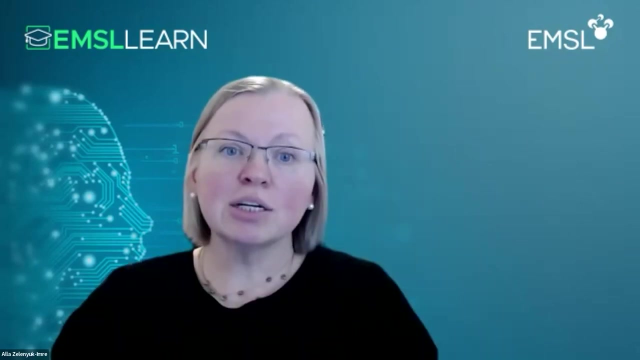 So we just use the raw samples and perform the analysis. We don't do any sample preparation or quoting of the samples. OK, Alla, does the SPLAT measure only the volatile fraction of the particle? No, we are measuring both volatile and non-volatile. 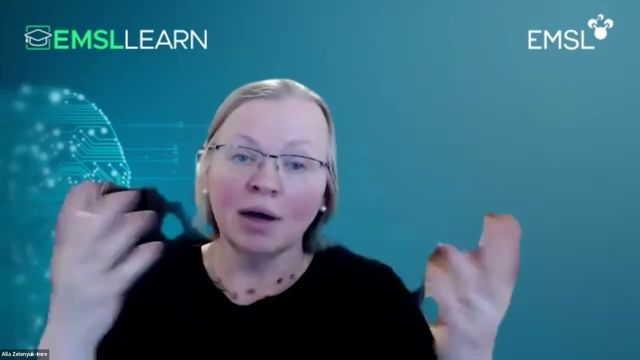 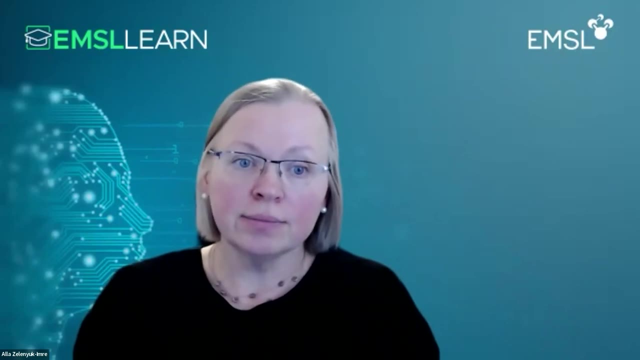 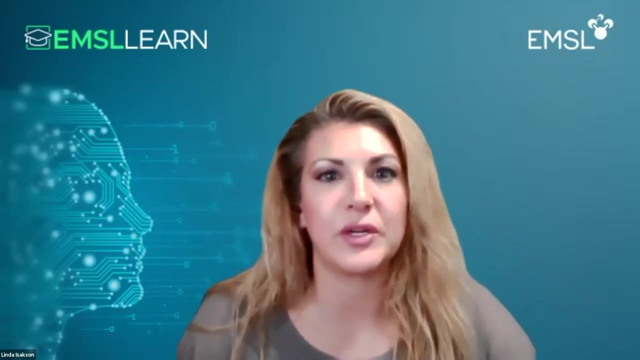 fraction in each particle. So we could look at this volatile organic coating on top of soot particles or dust particles. We are analyzing both fraction in each particles. OK, This one doesn't have to a specific person, so I'm just going to throw the question out and see who picks it up. 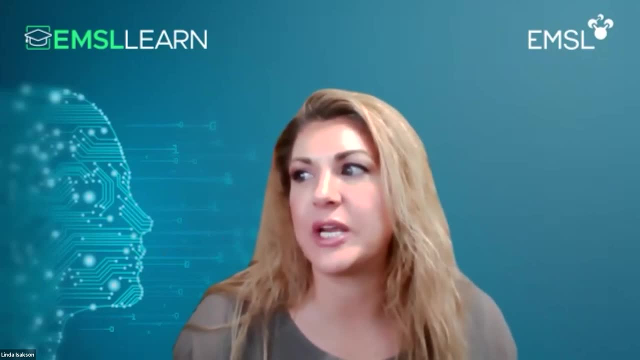 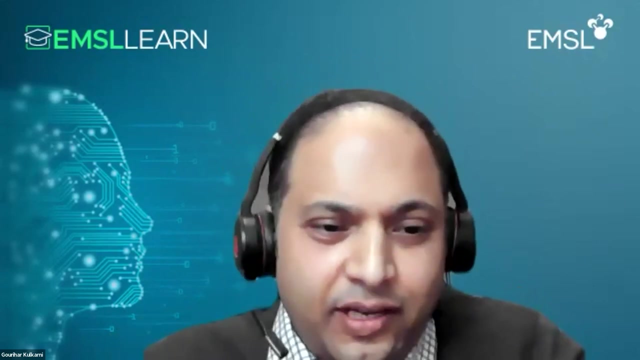 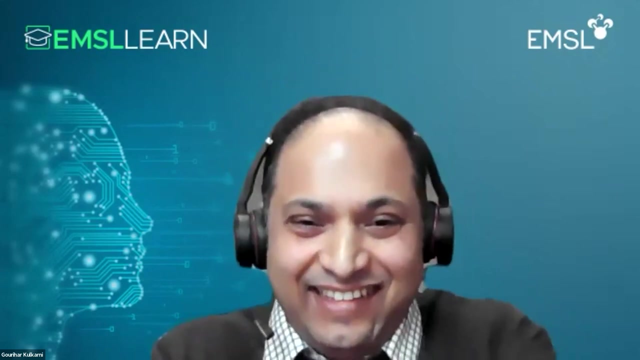 From a biological point of view, do you have any tips for characterizing signatures of pyrogenic aerosols? That means those particles do have some biomass burning elements attached to it. I think Alla's SPLAT. I think it's a powerful instrument. 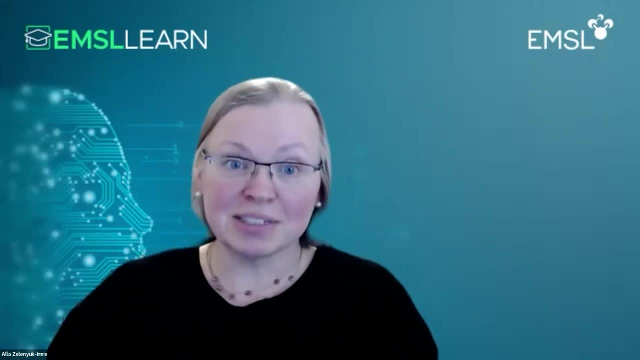 Yes, Both me and Swaroop have a lot of experience analyzing particles produced by biomass burning, both after long-range transport and collected from local fires. We are looking at the very complex composition, viscosity many of them as the star walls- optical properties. 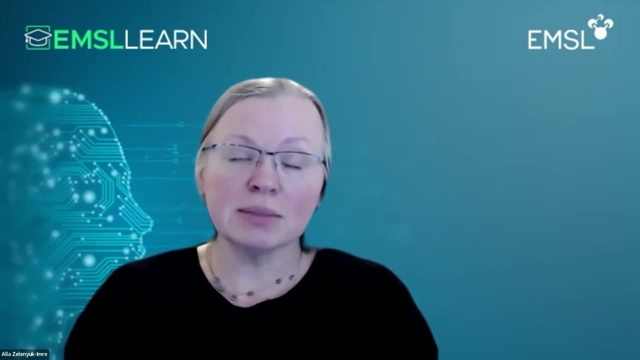 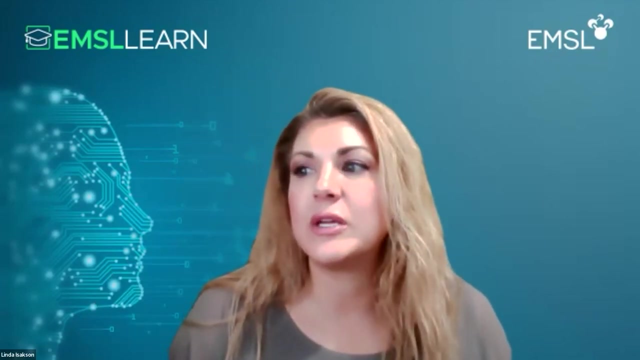 And we have both signatures for particles- biomass-generated particles, which carry signatures of primary aerosols, And also secondary organic aerosols, which are associated with biomass burning sources, And they have significant differences in the mass, spectral signatures and composition. OK, Here's another one that doesn't have to a, it's actually 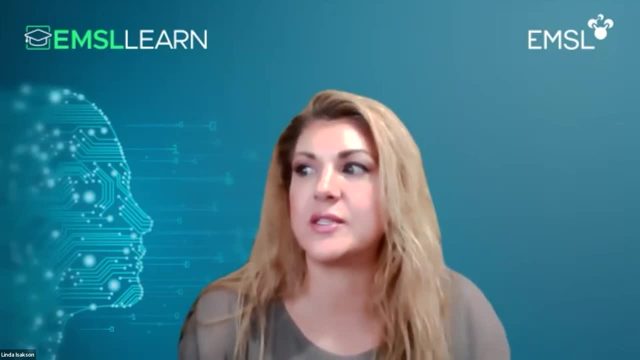 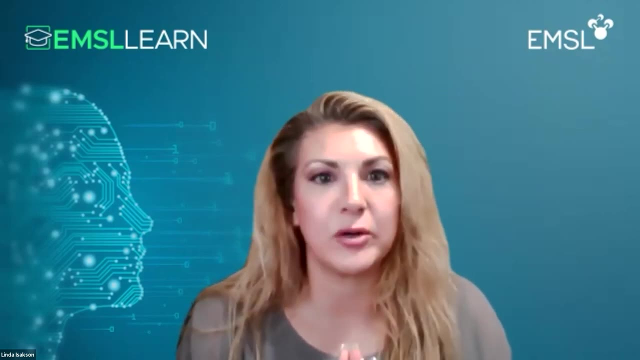 a series of questions that is not for any particular person, So there's three questions in this one. What is the typical output of iodine? How do you do that? Many of you have already asked about iodine. It's a breaking-down process. 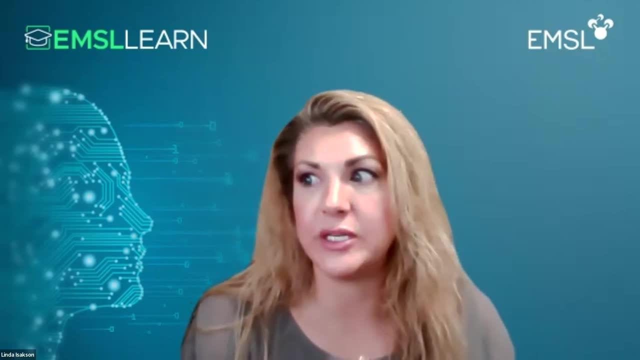 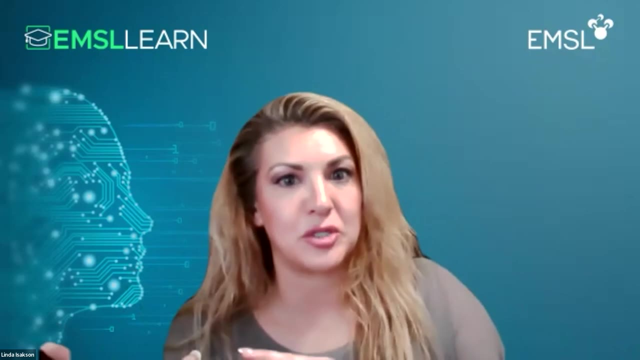 Does it go through MAC, the ideal ICRs that go through MAC speck. Can this processing be automated for high throughput And is there a similar pipeline between the EMSL offline droplet assay and the MS instruments? And I can repeat those if you need. 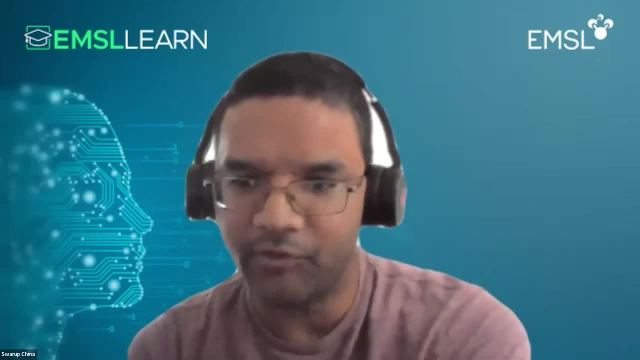 So I can brief answer the ICR part because, first of all, it's not, I'm not an expert. There are specific people that have done those experiments. So I appreciate your time and thank you for your иs And thank you for your time. 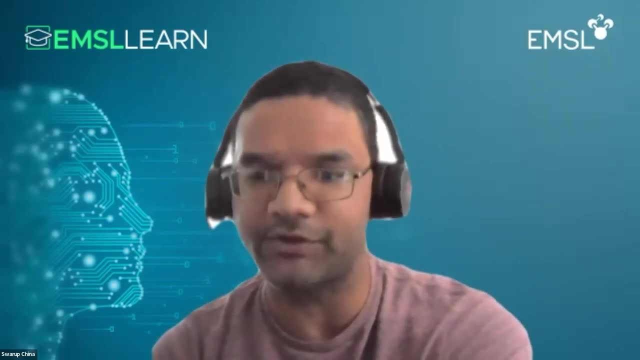 I'm very happy to be in the background And thank you for the discussion. I hope everybody will have another question. OK, Thank you very much. Thank you, Thanks for your attention. Thank you, instrument So they have more expertise on that. But for 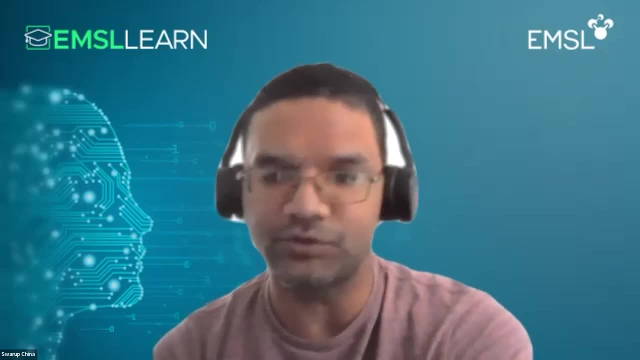 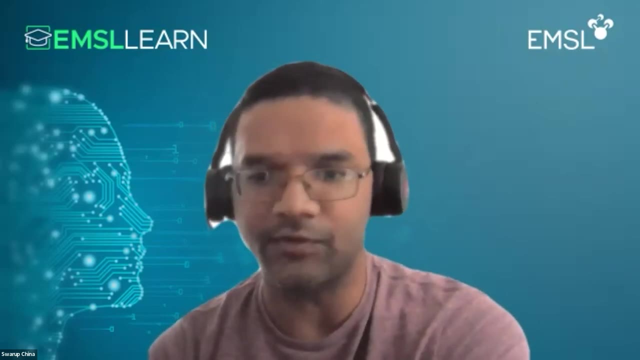 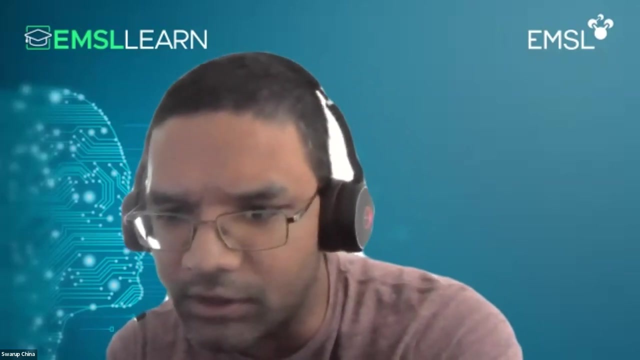 example, nano, this instrument that can go to the ICR instrument, And but there are also the auto sampler that use in the ESI mode, I guess, and that can be used for high throughput analysis, is in the direct infusion, And the second 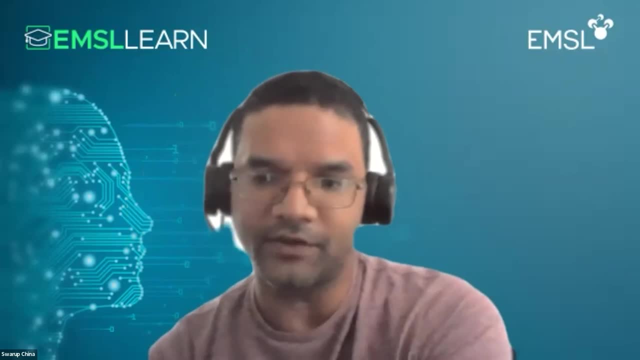 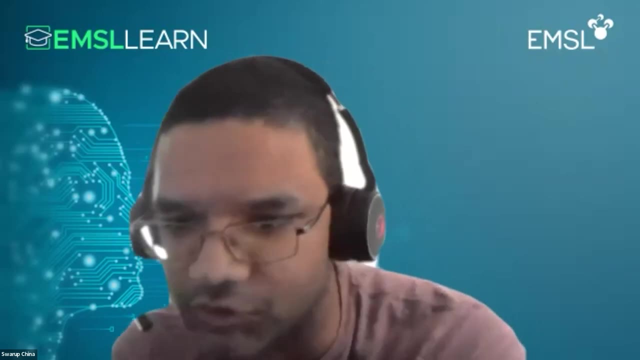 question is: can this person automated for high throughput? Yeah, so that was the. there is a automated auto sampler method that can go with with the ESI, the ICR instrument, And it's a similar pipeline between the end. so offline doc letters and MS. 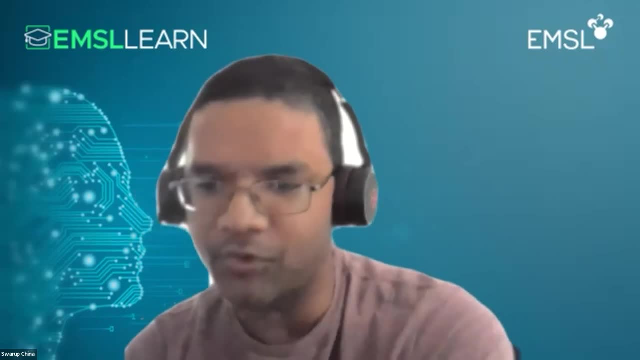 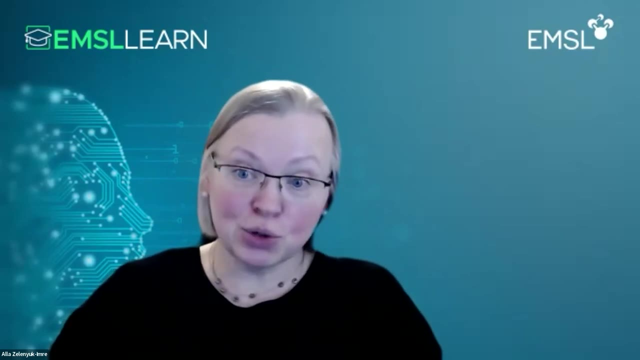 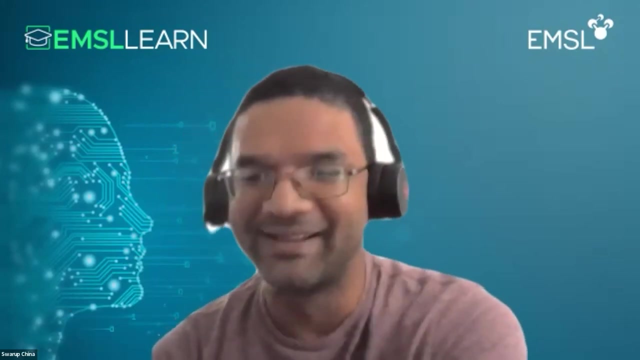 instrument. I'm not sure. Do you know what? I think it was the latest clarification that ICR it's ice crystal residuals. So it was. Oh, it's not. if I say okay, sorry, nevermind My bad. So is there a similar pipeline Or? 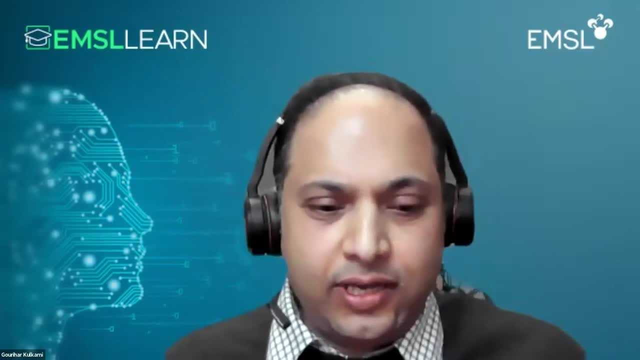 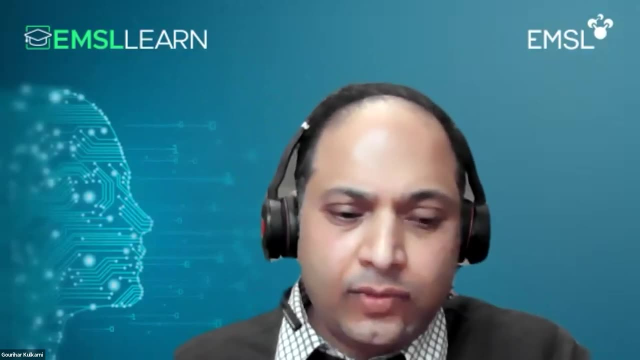 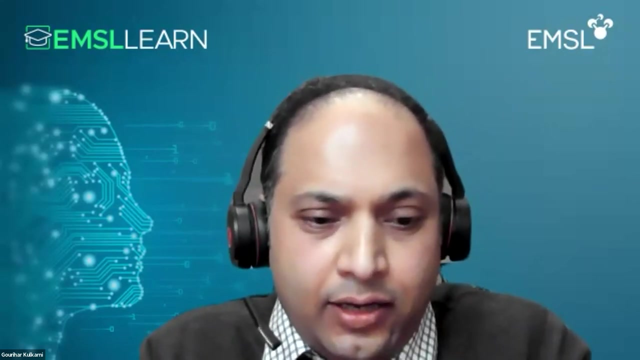 Yeah, So the ice crystal residuals can be transported to the, to the splat And also in a paddle. they can be also collected on a grids for further morphological analysis And currently we are in the process of deploying the whole operation autonomously. So basically, the chamber, PC VI and further. 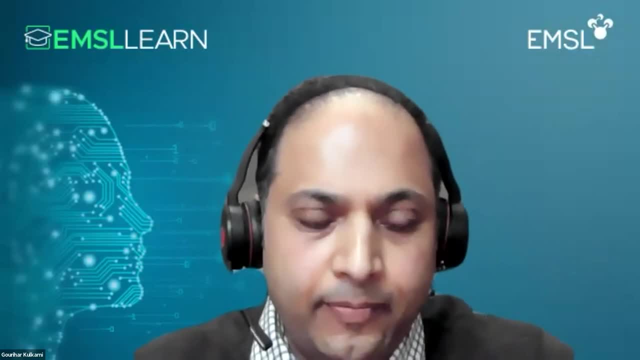 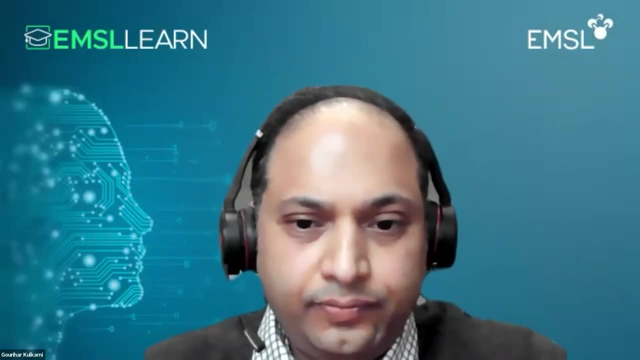 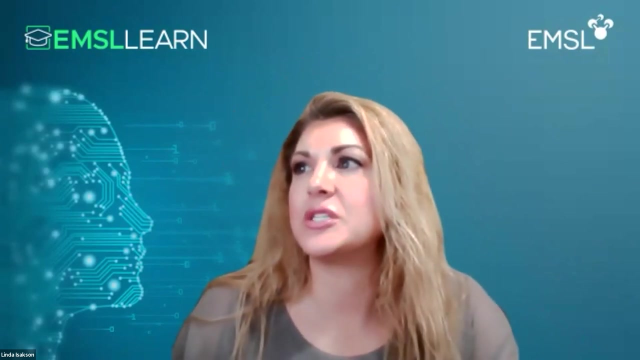 downstream instruments you can run continuously. It's not tested, but we have, our design is ready for that, to do it. It's possible. Okay, we have a few more minutes or a couple more minutes, So I'll see how many more questions we can get to Allah, or Allah, Let's. 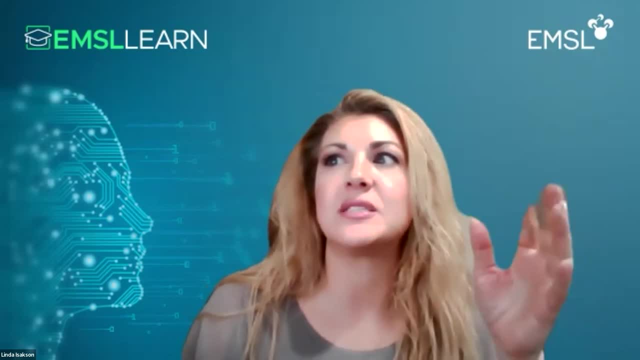 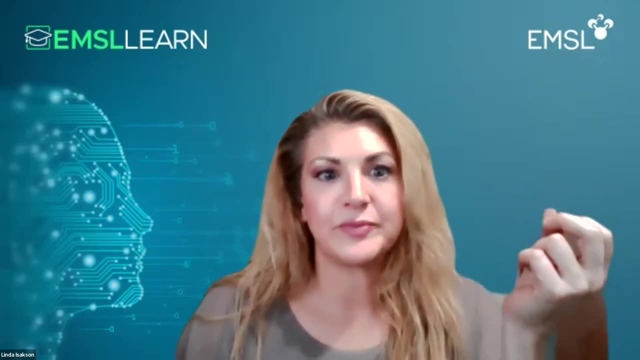 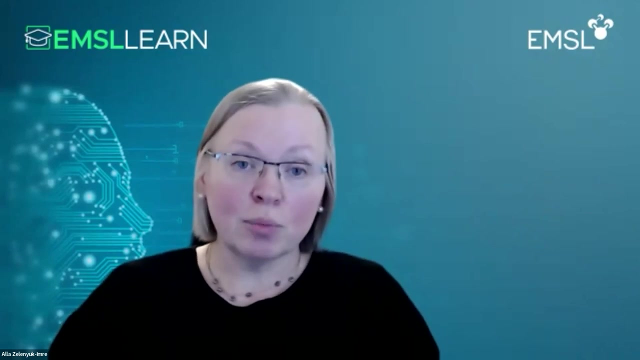 do So is the mini splat? Is it quantitative? How do you deal with, deal with information on millions of individual particles? So the instrument is quantitative And to achieve this quantification we correct for size and composition-dependent transmission efficiency and employ. 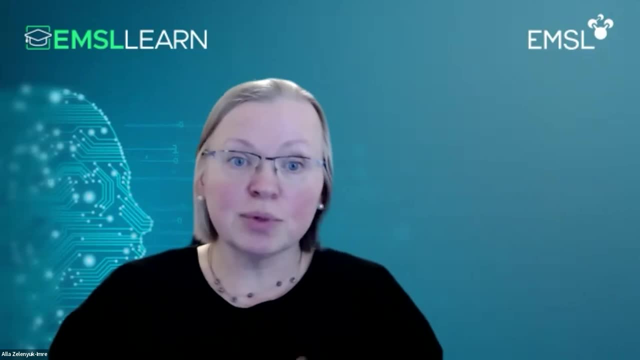 this multidimensional, single-particle characterization I was briefly referring to, And indeed during typical experiments, especially during field campaign, we are obtaining information on millions of individual particles. But to deal with it we develop very special software which allows us not only to visualize, 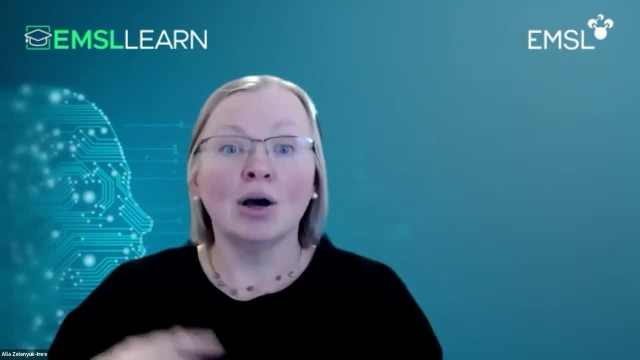 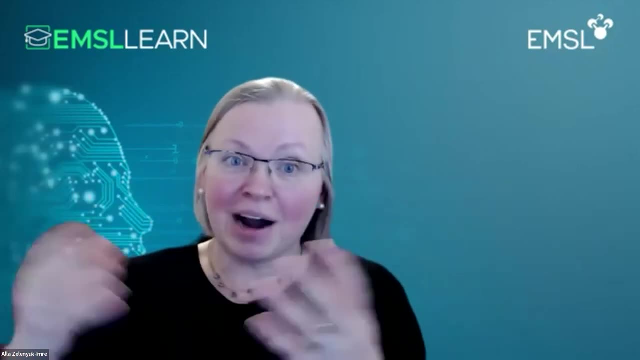 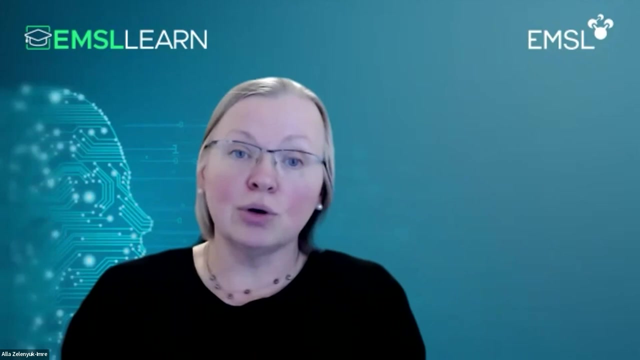 different particle properties, but also to explore correlations, anticorrelation, causation, And I had the screen captures. You could pull out only particles in Arctic in the cloud which activated as cloud condensation nuclei and compare them to those which did not. 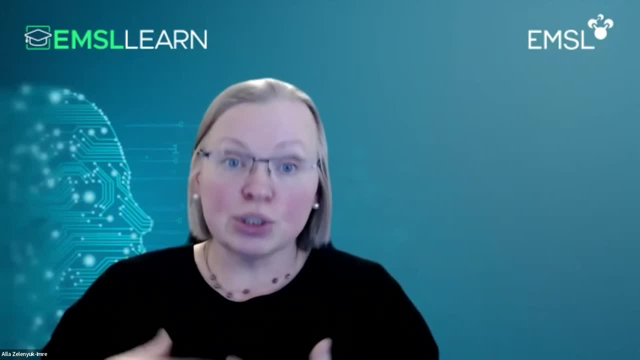 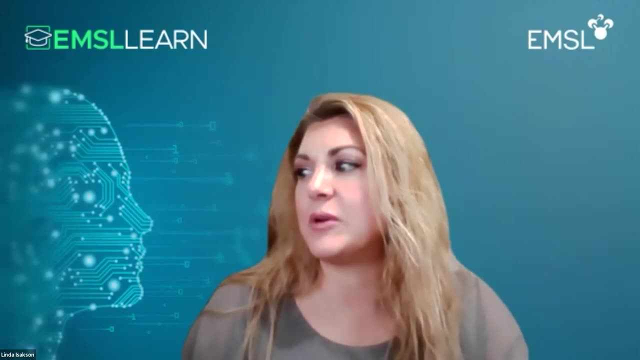 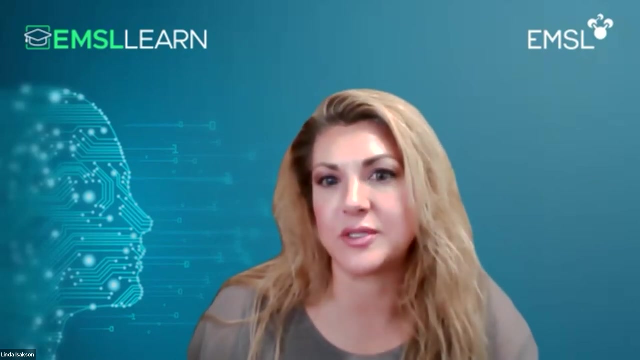 So it relies on very special approaches to visualize and analyze data. Thank you Great. We have one more question, Or I think we have time for just one more question And it's got to be quick. So, GK, how do you collect and analyze ice crystal residuals? 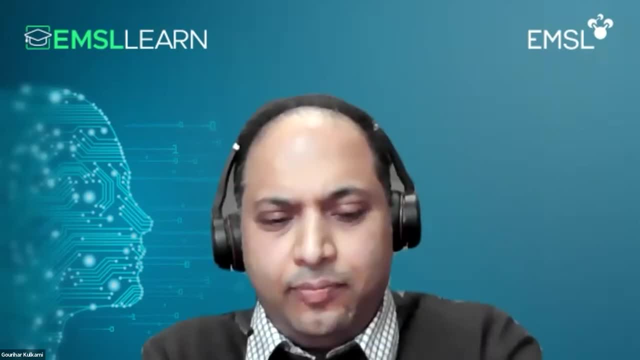 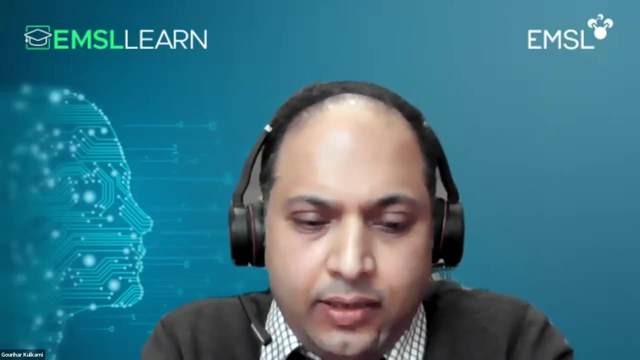 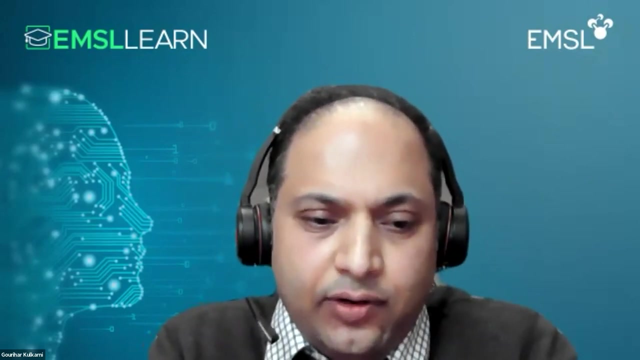 Did we already answer that. I can briefly again mention this. So there are multiple approaches. One is you can continuously keep collecting or sending them to the mass spec, like a la the SPLAT, Or you can collect Collect them on a grid. 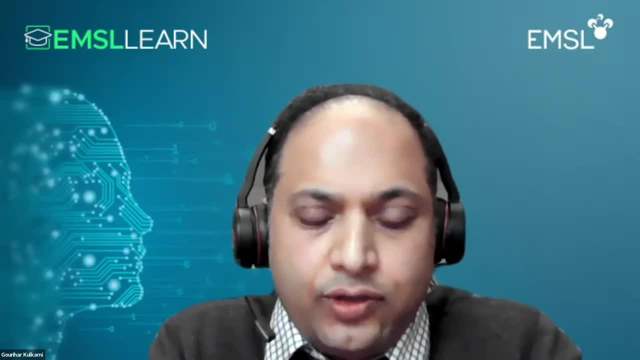 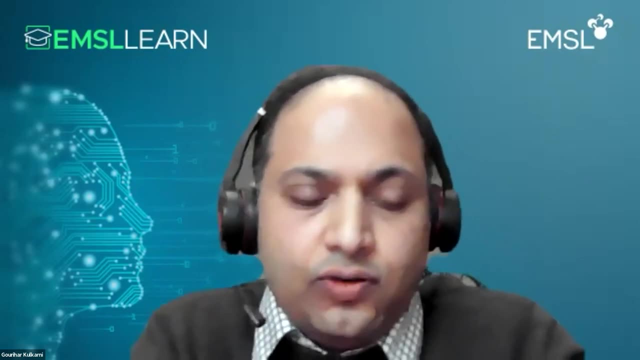 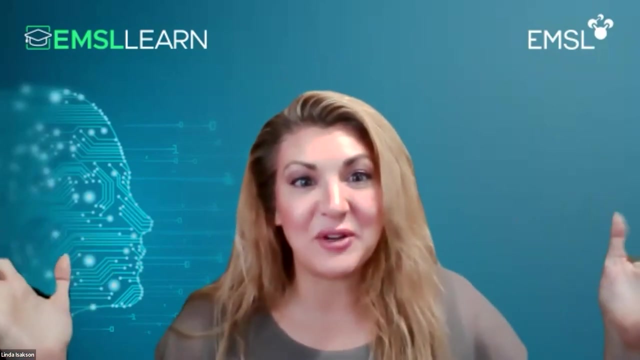 And then you can analyze the grids later. So you can do both the online and offline analysis of the ice residuals, depending upon the application and the research question. All right, Well with that. thank you everyone for your time and attention. 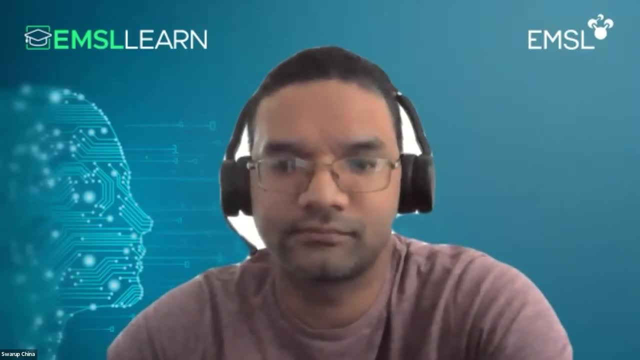 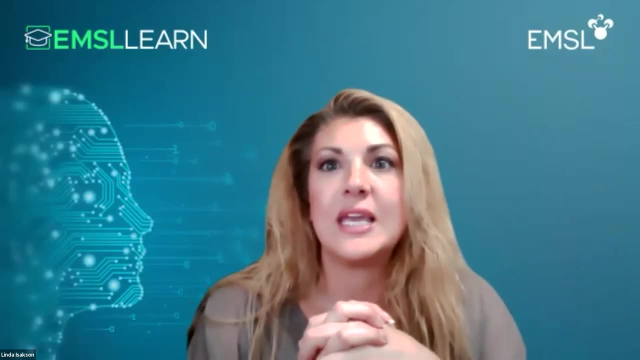 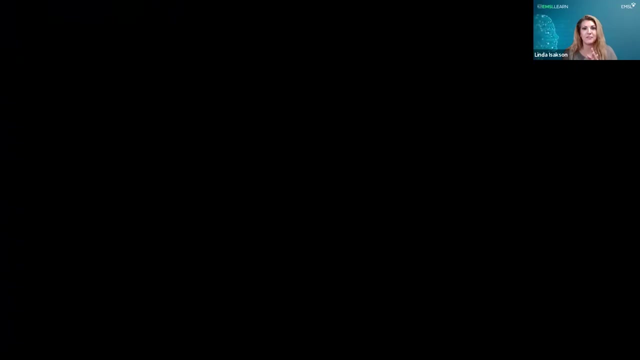 If you have any more questions, feel free to contact the panelists or contact us based on the information in the chat window, And we hope to see you at the February 9th EMSL Learn webinar on submitting a FICUS proposal for the JGI- EMSL FICUS. 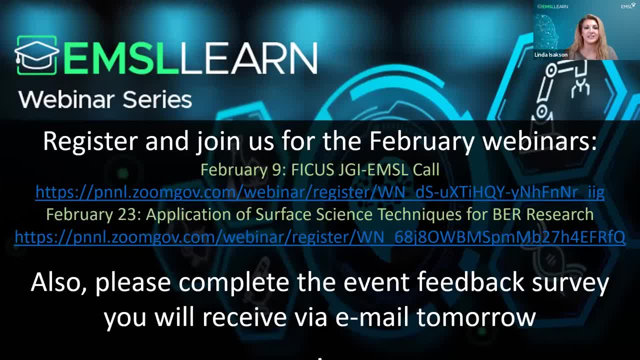 call. So thank you everyone. Have a great rest of your day.